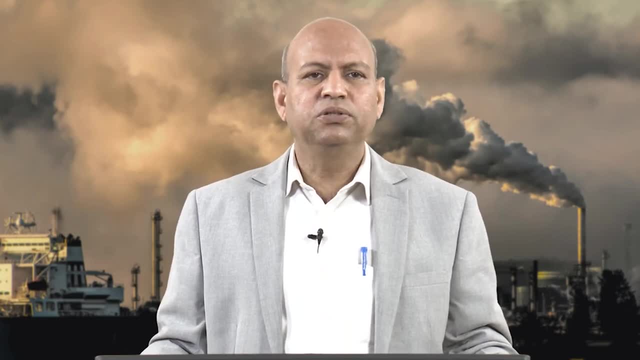 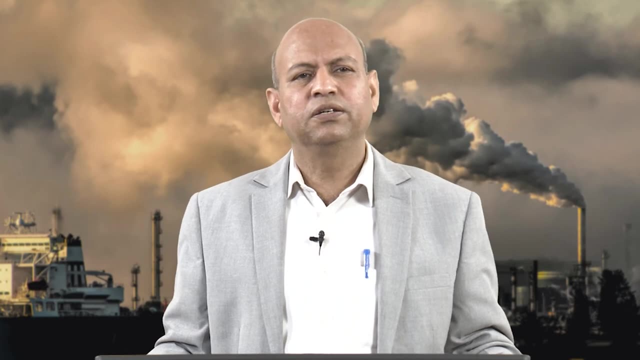 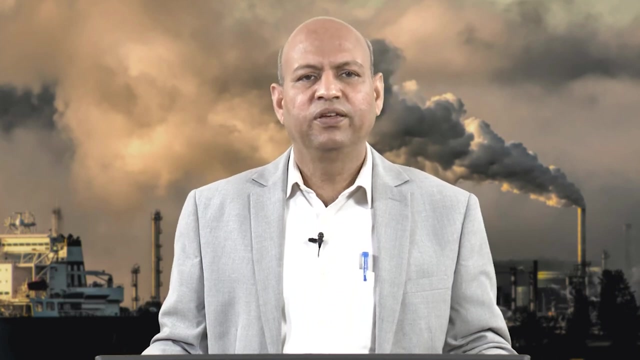 pollution through these controlling devices. Well, so in introduction we can say that this control of the air pollution is very important and in a most effective way. if you want to control the pollution, then it is better to control at the source itself, And one of these methods, which 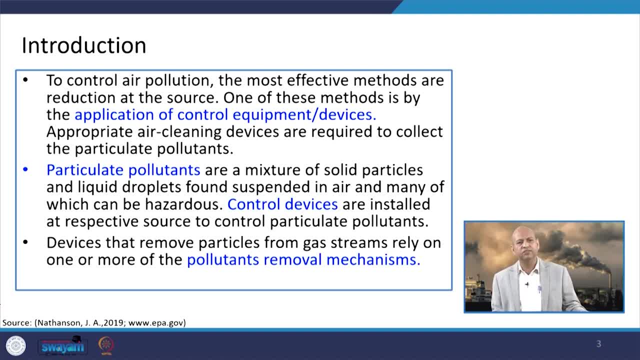 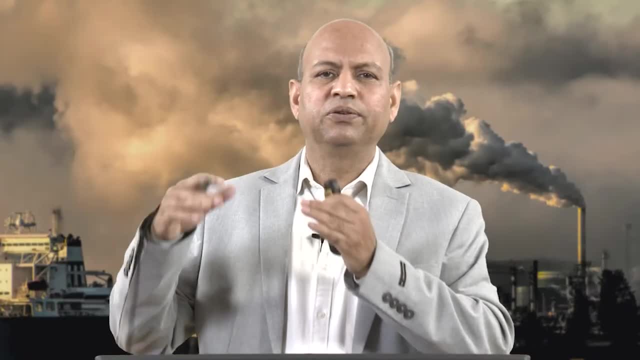 are prominent or effective to control the air pollution emissions is by the application of control equipment or devices at the source itself, and appropriate air cleaning devices are required to collect the particulate pollutants, Because whenever there are, number of pollutants are emitted, So as per the nature of the pollutant, 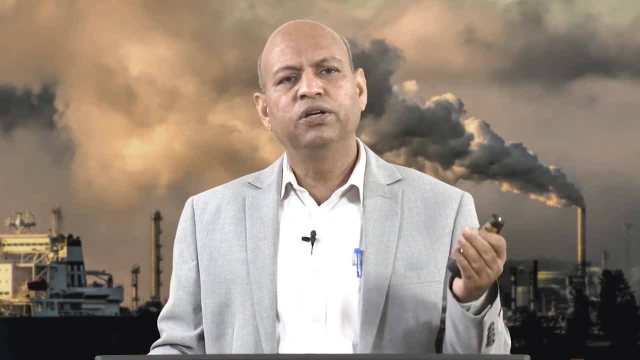 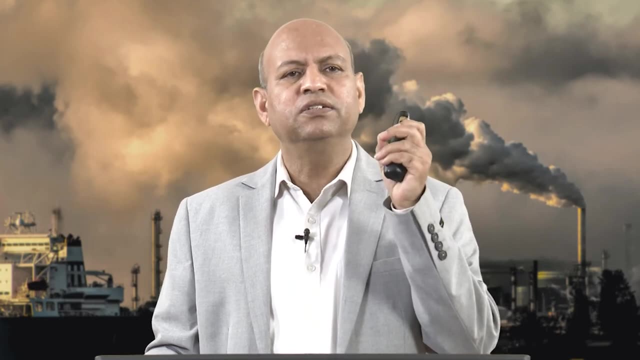 it is particulate pollutant or gaseous pollutant, we have to install some equipment or controlling devices. So today we will discuss about particulate pollutants: concentration reduction or control of the particulate pollutant emissions basically. So we will see how particulate 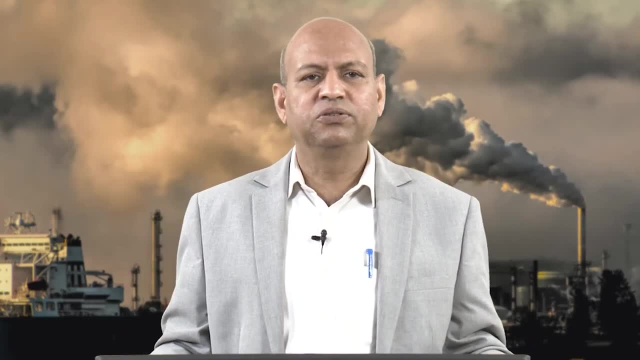 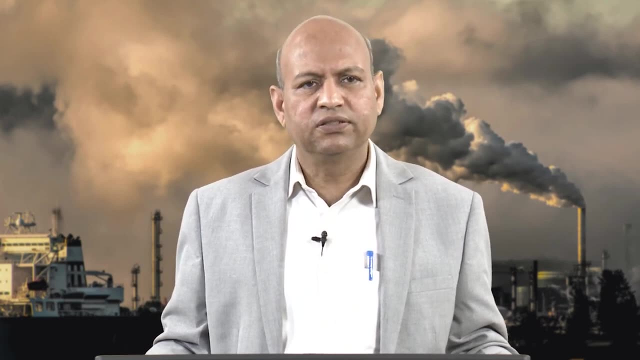 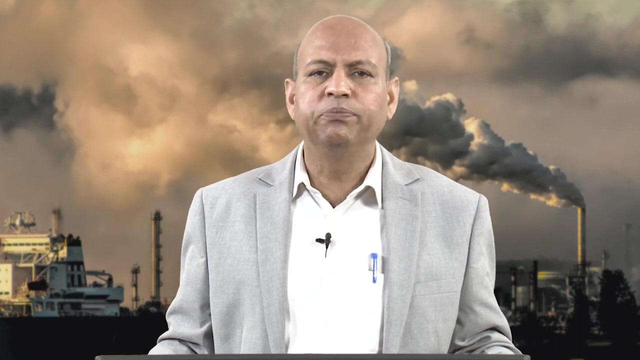 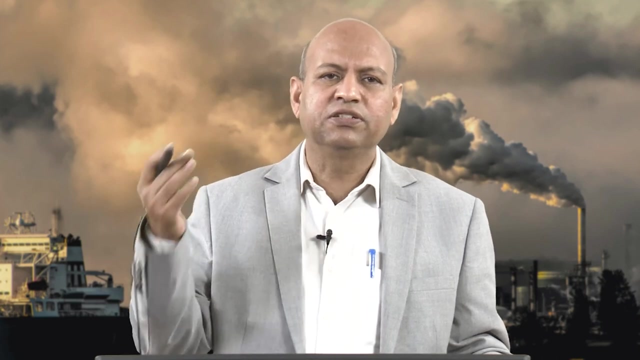 matters of different sizes or different densities we can control. So these control devices we will focus only on particulate matter concentration or collection, basically. So if we talk about, like different pollutants, removal mechanisms which are used for removal of these particulate pollutants, then basically we list, like gravitational settling or centrifugal. 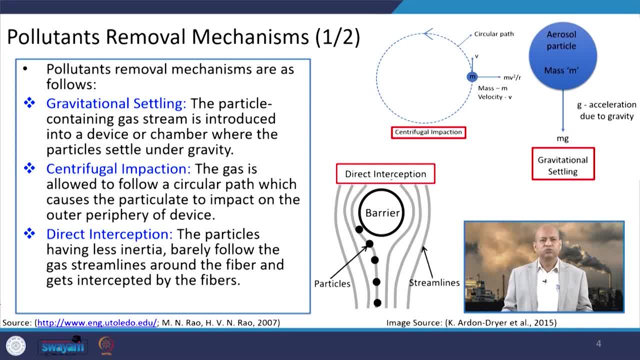 impaction or direct interception, those kind of things. So in gravitational settling- basically only the gravity- it acts like there is a mass of the aerosol or particles. So gravity pulls and it settles down because of simple gravity. Then we can also mimic this. 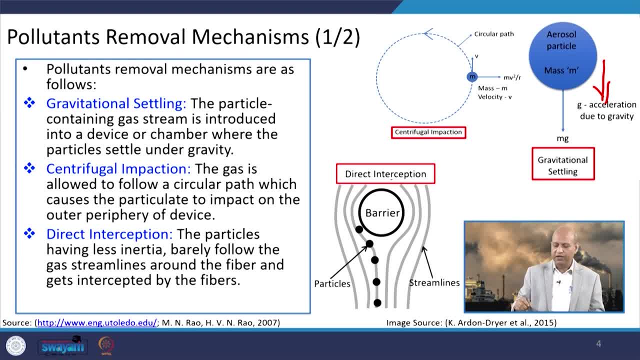 pulling force or gravitational force by creating centrifugal force. So if we rotate by some device, the particulate matter, then there will be centrifugal force and it will strike to some surface and then there it will lose the velocity and it will be collected. 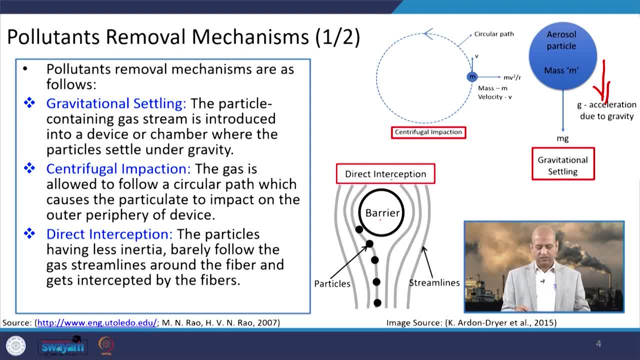 Or we can also do like impaction through barriers. whenever we change the course or this direction of the flow, then what happens? like these particles which are having mass, So because of the momentum, they just go in the straight line. they not quickly change the path, like the. 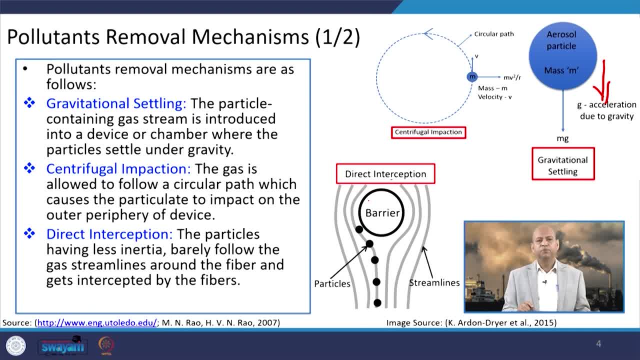 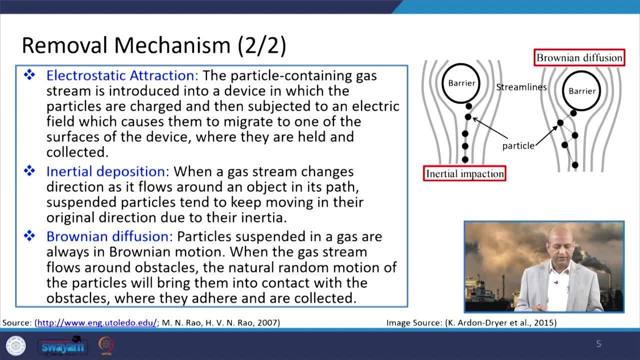 gas. so they will have the tendency of striking to the particular that barrier and then again they can lose the velocity and they can be trapped or collected. Then there may be another way, like electrostatic attraction. electrostatic attraction force is created by kind of ionization. So we have different kind of 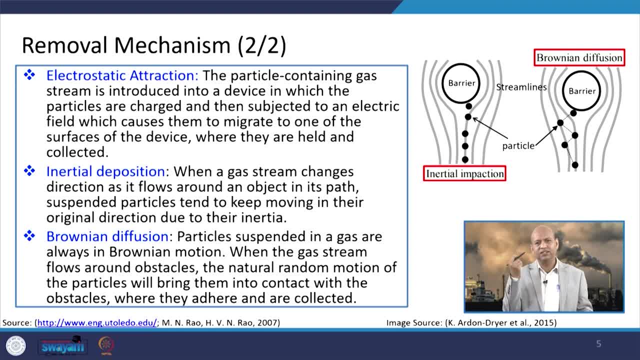 field, Sir, where particles pass through, so they get charged, and then on the opposite charge, there is one device where they are collected. then they lose again the velocity and slides down. Inertial deposition can be there, as these baffling kind of things may be there, or Brownian. 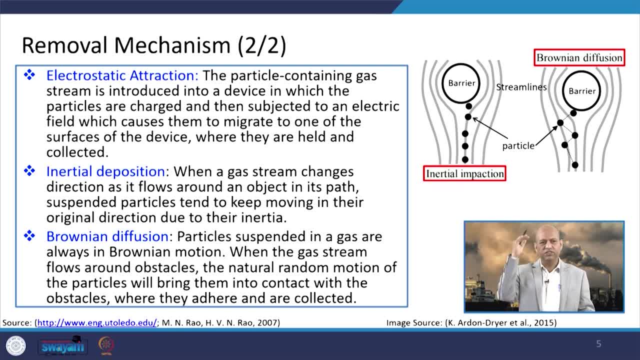 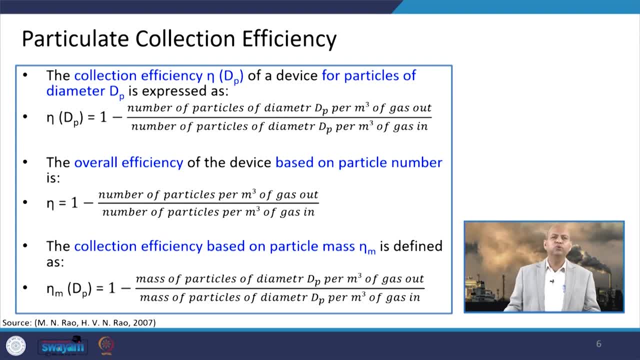 diffusion. so ultimately they get attached to some surface and slide down or get collected at the hopper at the bottom. So if we want to collect, then as an engineer we also want to know what is the efficiency of collection. So in a general we can say like this: efficiency related to a particular, let us say, diameter. 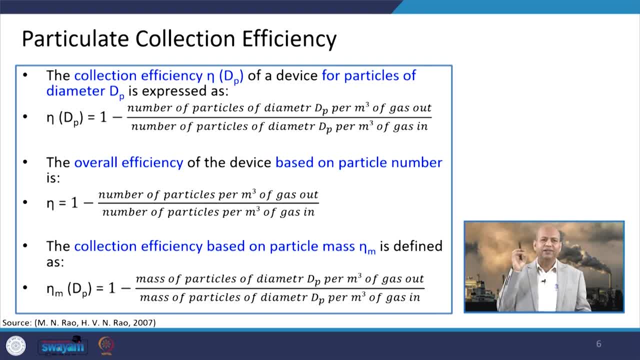 of particle dp. if we want to calculate the collection efficiency of particulate pollution of the diameter dp, then 1 minus number of particles of that diameter dp only per cubic meter of the gas. So going out divided by the number of particles of diameter dp only per cubic meter in the 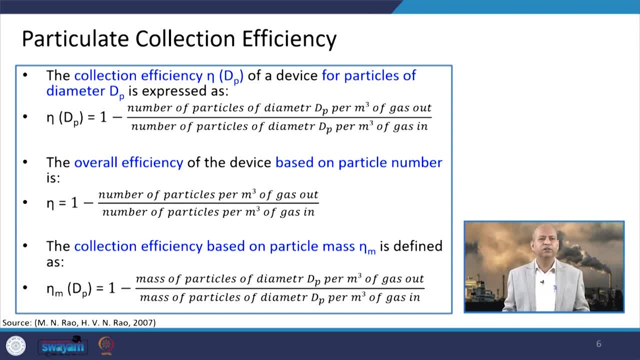 flow gas coming in. so that is the simple relationship. If you want to just the overall efficiency, then rather than this particular diameter, we consider number of all the particles, so number of all the particles going out per cubic meter- remember this- and number of particles coming in, so that division and deducted from 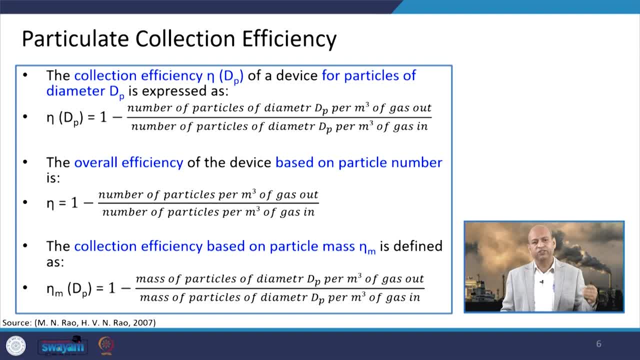 the one. so that is the particular efficiency of overall efficiency. If you want to see the collection efficiency based on particulate mass, this eta M mass related, then it can be defined. it like: defined like: mass of particles of diameter dp per cubic meter of gas going out divided by the mass of particles of diameter, dp per cubic. 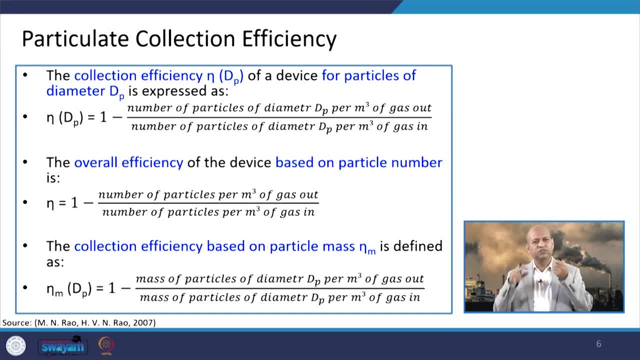 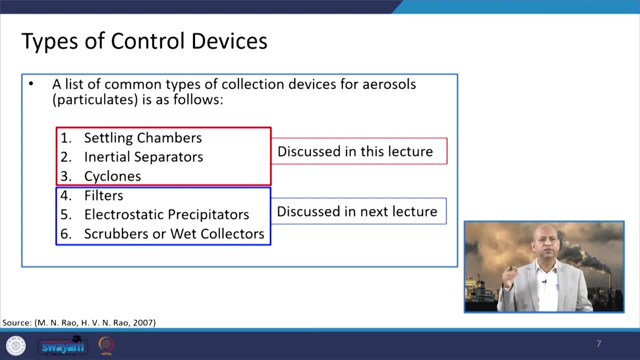 meter of gas which is coming in that device. So that is overall efficiency related, related. So NR interesting. so after this I will finish話 with you All the screaming recorded relationship which we generally use because it will be used later on to calculate the 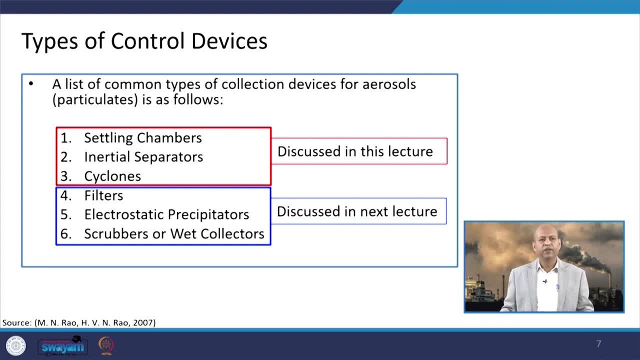 efficiency. that is why we discussed just now about this. Then if we talk, what kind of devices are there which are available in industrial pollution control? so the list of common types of these air pollution control devices or collection devices of aerosols or particulate matter is like settling chambers or inertial separators. 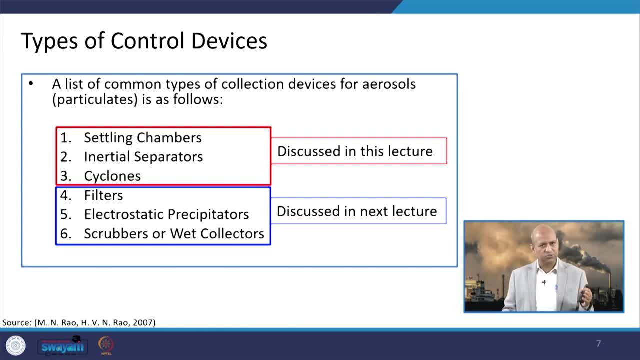 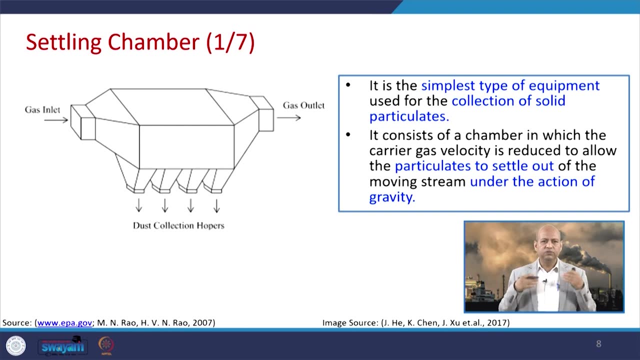 or cyclones. these three types of devices we will discuss today. Then there are like bag house filters or filters, fabric filters, electrostatic precipitators or scrubbers or wet collectors. they are known, as we will discuss in the next lecture. So if we start our discussion on settling chamber, that is the simplest device, basically. 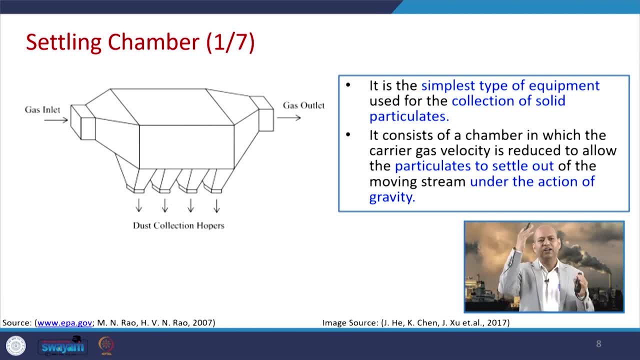 you can say this is simple: chamber length, width, height. So this kind of device- So there is inlet gas length Leaden by pollutants, goes into this and it comes out of this particular outlet. So there is a distance, this length, L. you can say this has to be travelled by this gas particles. 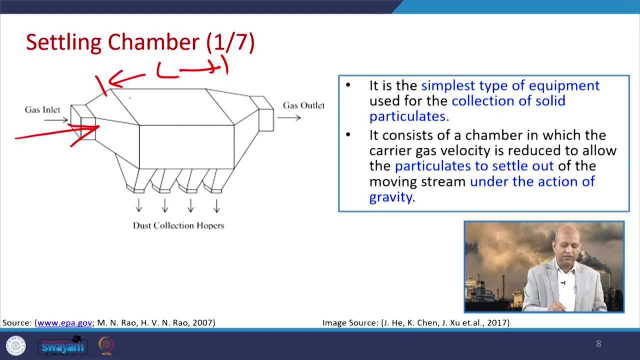 particles are there in the, this dirty gas, and this particle has the mass, so it has tendency, due to gravity, to go down. So when it travels to this distance, this should be of such a speed or velocity that this particles comes down before going out through the outlet. 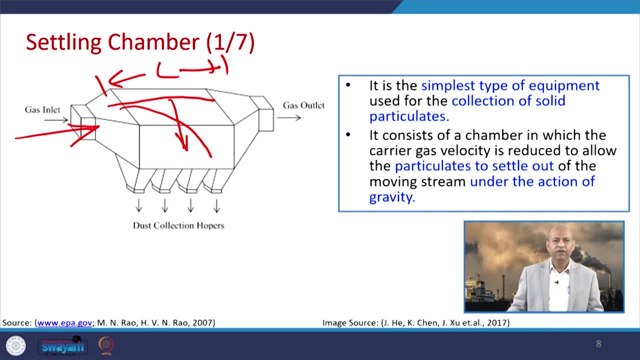 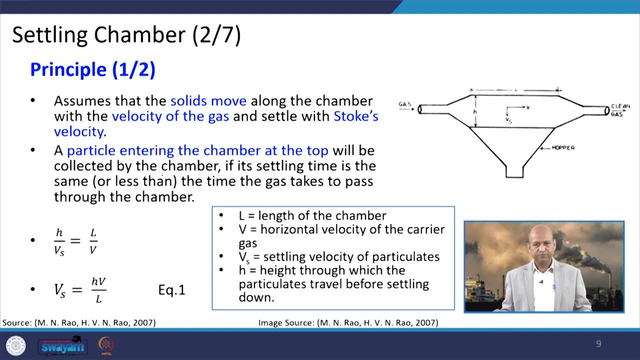 That is the fundamental thing, very simple understanding we have to develop that it should be removed. only then it will come down and we will remove from the hopper. So you can see here like this is the chamber, settling chamber- of the length, L and height. 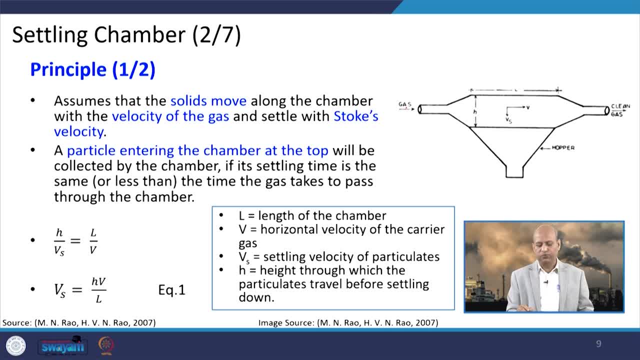 H, and this gas which is full of these particulate matters is going inside and this velocity of the gas is V, simple V, Okay. Okay. So these particles which takes it down is Vs, right. So this Vs should be such that with this Vs, this height will be travelled this length. 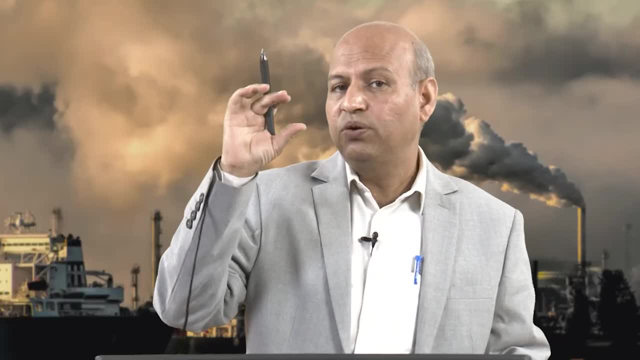 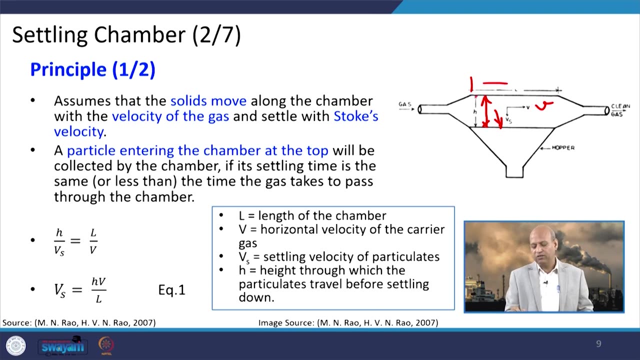 of the height. for that particle, this path is of the length height And this gas, the path is length L. So with V, when this particle comes to this stage, this should basically come down So that S divided by Vs equals L divided by Vs. 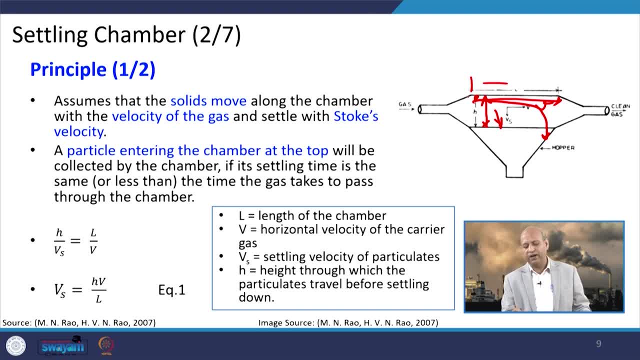 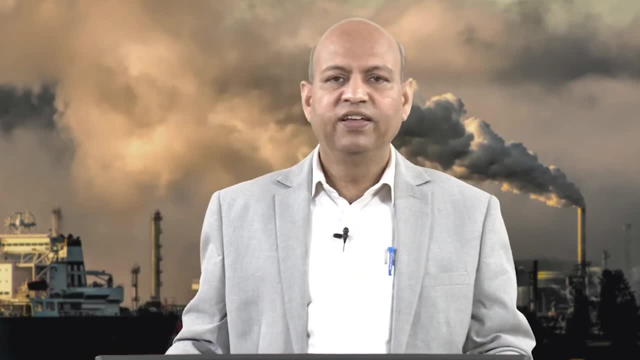 So the time taken by one particle, when which it travels from this point to this in the horizontal direction, in vertical direction, it should have the velocity of Vs and it should come down So that particular diameter of the particle we have to design for that, how this Vs can. 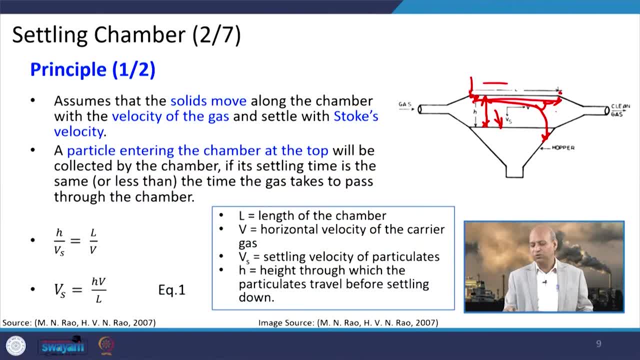 be achieved so that it does not go out with the this dirt, this dirty gas. rather, it comes down, And this L is length of the chamber. as you know, V is the horizontal velocity of the carrier gas and Vs settling velocity of particles, and H is the height through which this you 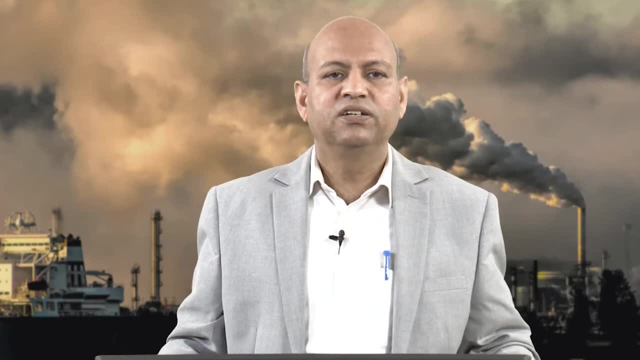 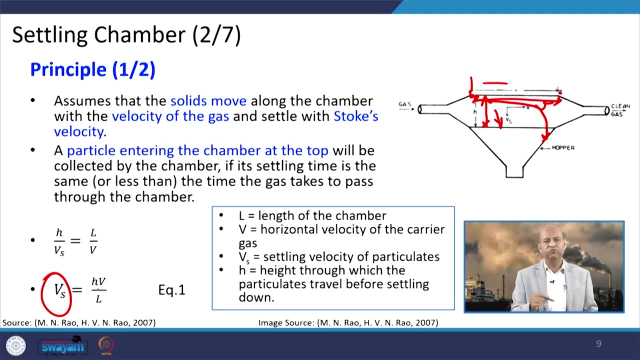 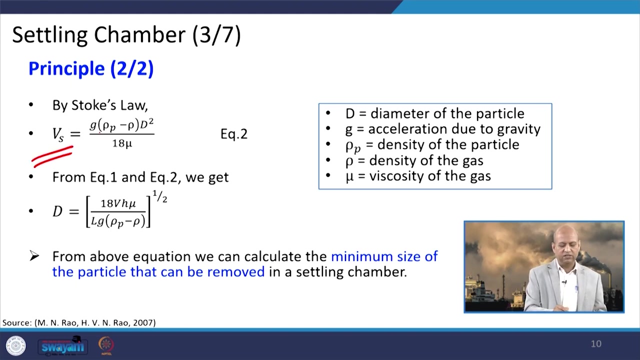 know particulate matter, travels following the stocks velocity, right. So this Vs is nothing but this Hv divided by L, So that way we can calculate the velocity. This stocks law, you know, with the, you can represent it by this Vs: g into rho, p minus. 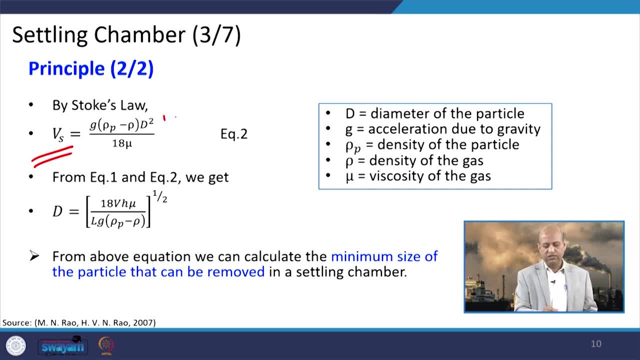 rho d square divided by L. Okay, So d is the diameter of the particle, g is acceleration due to gravity. as you know, rho p is the density of the particles and rho is the density of the gas carrier. right, Mu is viscosity of the gas. right. 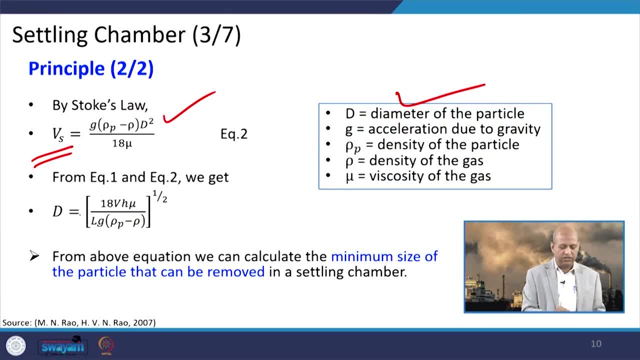 So when we, you know, determine d using this equation, so you can just play with it- and square root of 18, V, H, mu, divided by L into g, rho, p minus rho. So that way this is the diameter, which is basically the minimum size of the particle. 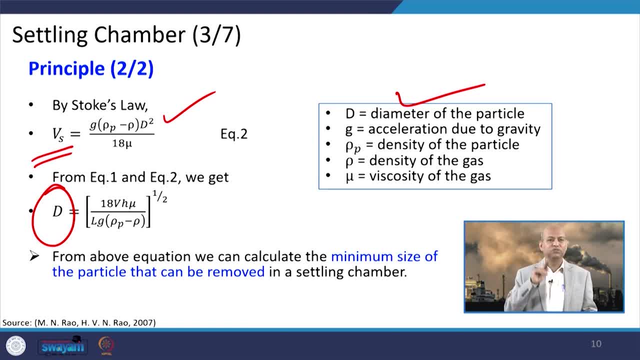 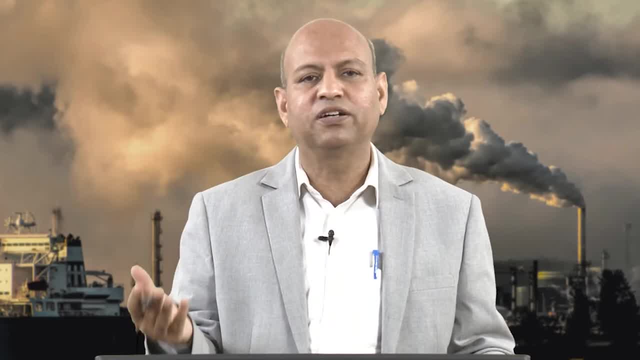 Okay, Which can be removed in a settling chamber. So this will decide that this will be the minimum of size. beyond that size they will have more than Vs, So they will automatically come down, but this is the minimum size of the particle, which will be removed almost completely. 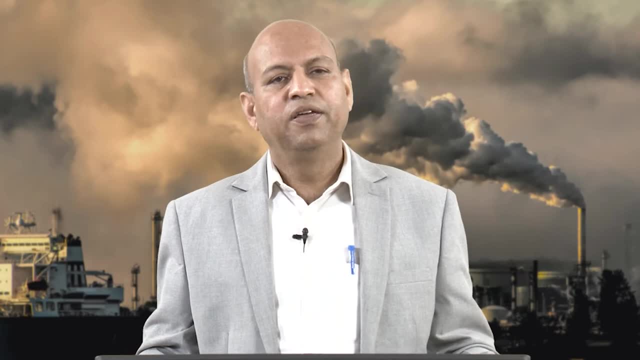 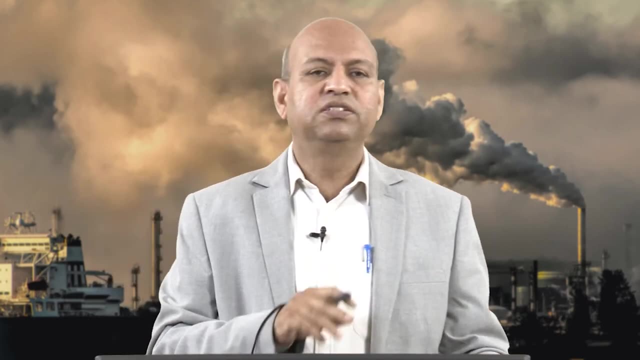 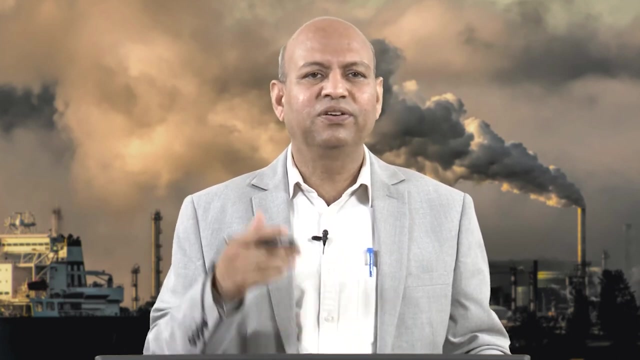 So that will be the design parameter for settling chambers. like particulate matter of different size exist in the exhaust gas, So we have to design the settling chamber to remove these particles, which are mostly coarser particles, Coarse size particles, and these are, you know, used for cleaning of the gas when it is passed. 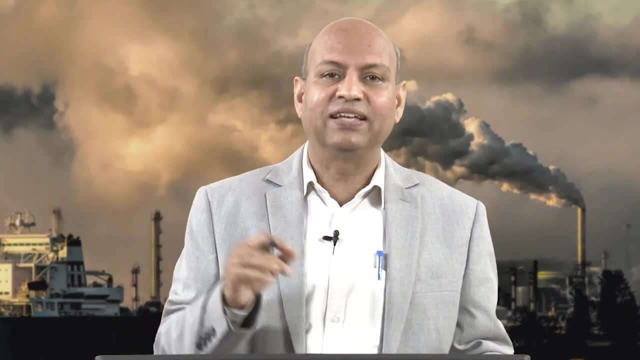 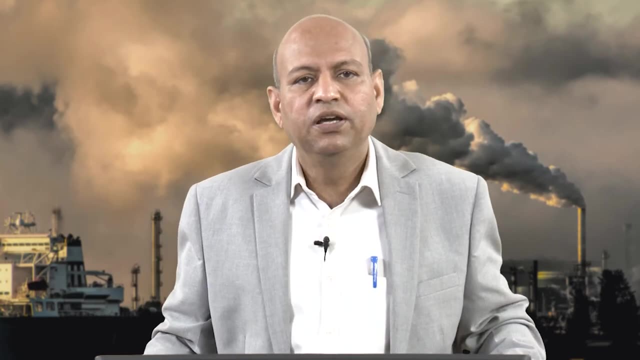 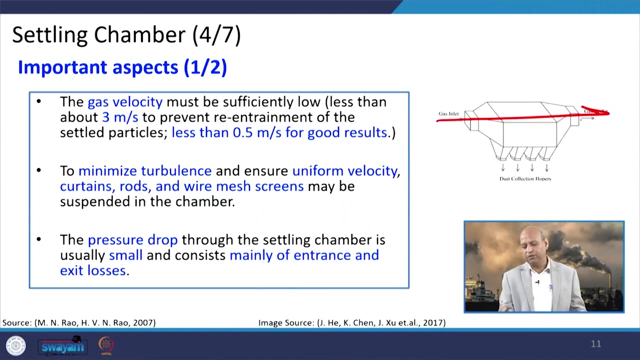 through other instruments, so that on those instruments load is less in comparison. right, Then there are certain important aspects, so like, for example, the gas velocity must be sufficiently low. if it is more, if it is speedy, then short circuiting will be there and gas will directly pass through this, taking the pollutants out. 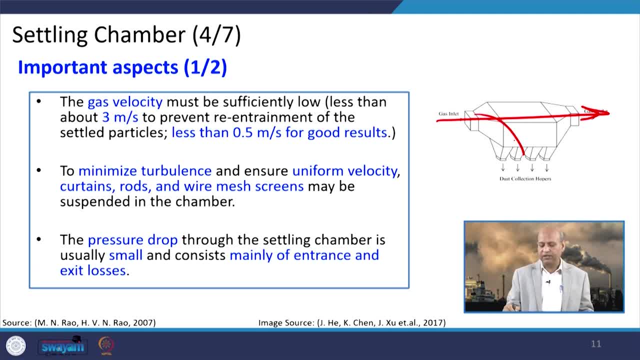 So that is not effective. We want to collect Those particles, so this gas velocity must be, you know, slow, or it should not be more than 3 meter per second, and so that it can, otherwise, you know it is speedy, it will short circuit. as well as resuspension of the dust, particles may also occur because of this high 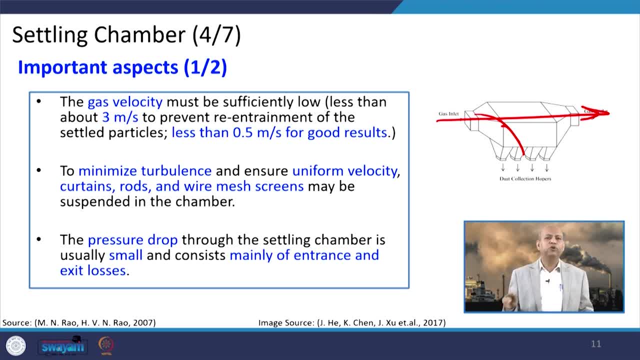 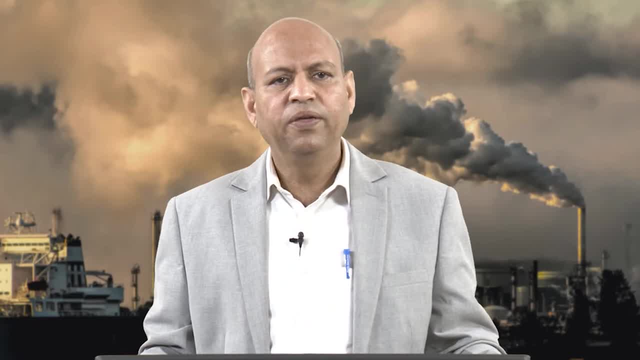 speed, So that we have to avoid less than 0.5 meter per second is the, you know, the velocity which gives very good results. So 0.5 to 3 meter per second. we have to maintain it Then to minimize the turbulence. 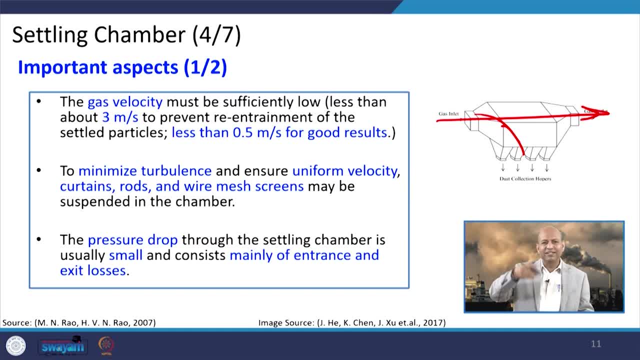 To ensure uniform velocity. you know sometimes you know curtains or rods or wire mesh, those kind of things can be applied right by suspension so that this inertia kind of things occur and the pressure drop through the settling chamber is usually small, not much. not much and consist mainly of entrance and the exit losses only. 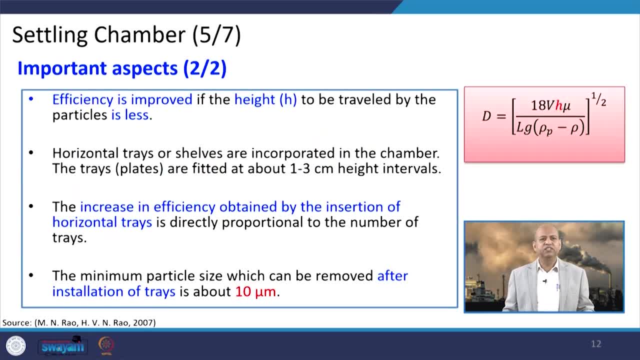 So that way, it is very simple way. Then, if we talk about the efficiency, then it can be improved by the height. okay, improved in the height, So the terms of height as travelled by the this particle, when efficiency is improved if the height travelled by the particle is less, okay, otherwise there are other problems. 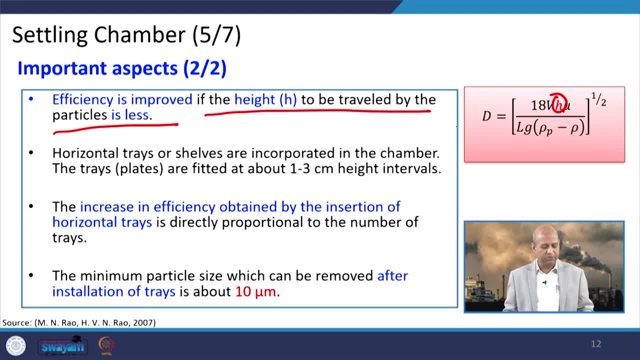 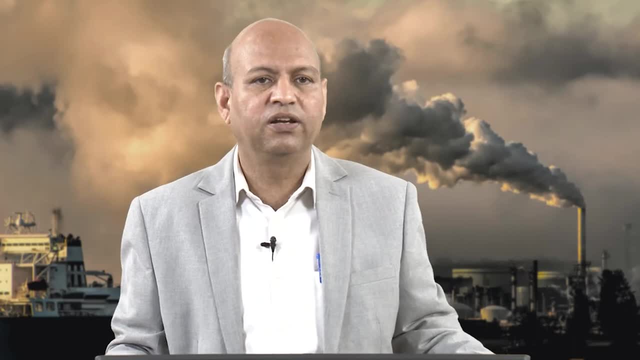 So this is less right. so diameter related height can be calculated. Horizontal trays or shelves can be incorporated to reduce this height part, otherwise there will be large height. So you can install more horizontal plates so that effective, you know, height can be reduced for several diameter of particles. 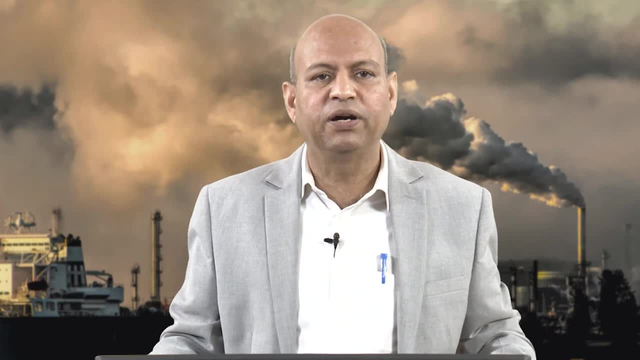 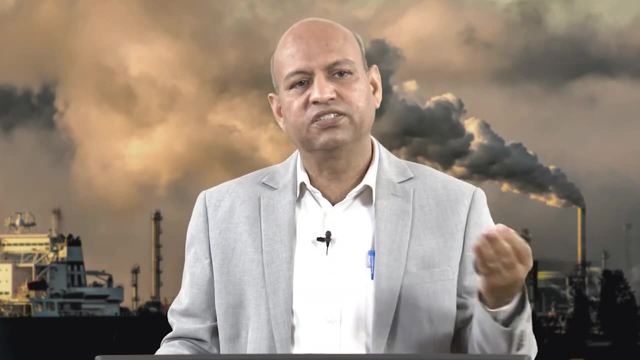 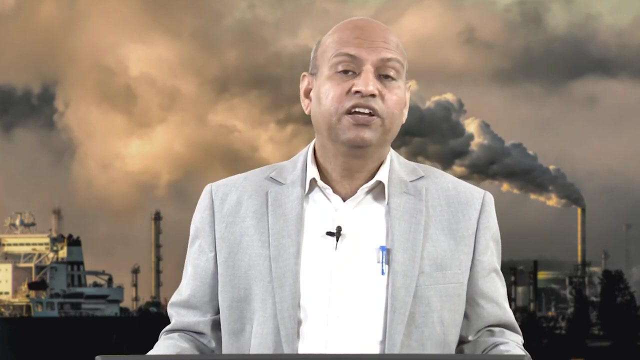 And to you know, this increase in efficiency obtained by these insertion of horizontal trays directly proportional to the number of trays. basically, that efficiency can be governed by the number of trays, And the minimum particle size which can be removed after installation of these trays can be up to 10 micrometer. otherwise, generally, it removes up to 40 micrometer or so. 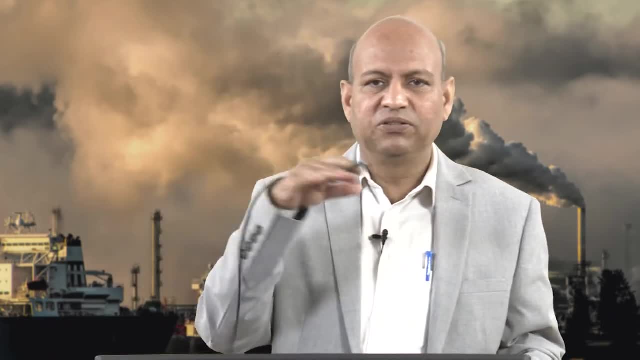 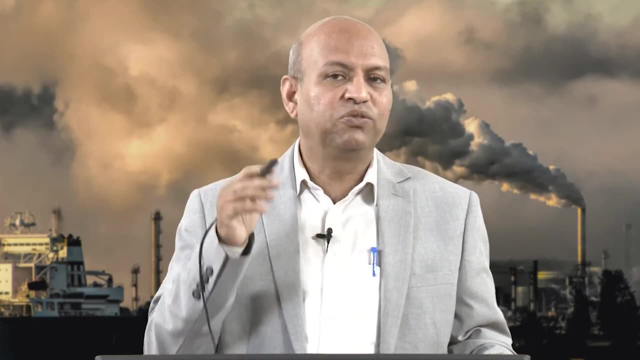 But by these, you know, manipulation of, you know this settling chamber through horizontal trays, etc. You can improve the efficiency in terms of the size of the particle so that you can remove even fine particles up to 10 micrometer, which is PM10 or RSPM- respirable suspended particulate. 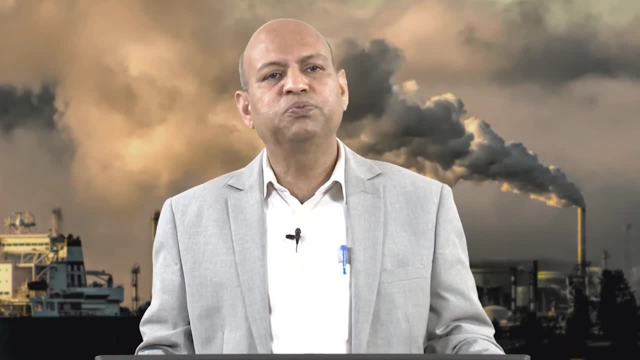 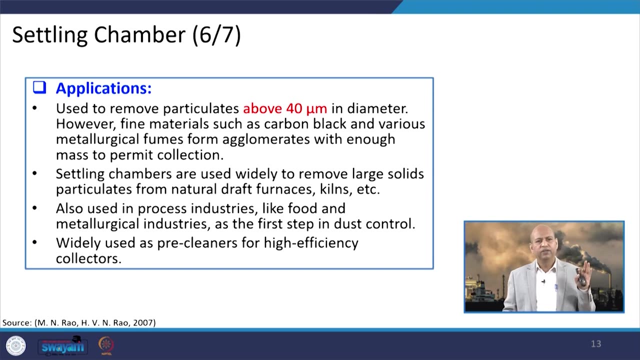 matter. So, as I said, you know, this is used for removing the particulate matters of size equal to or more than 40 micrometer. for that it is very good, And if you want to reduce further, then you have to apply certain those horizontal trays. 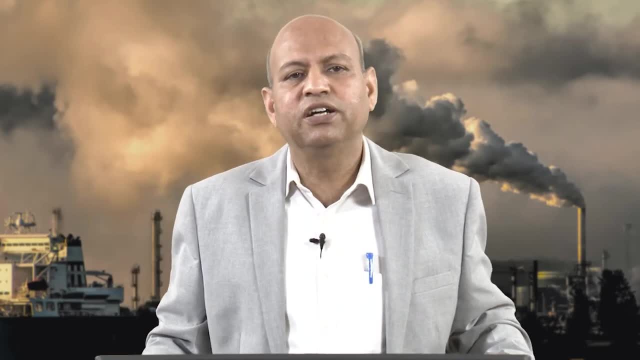 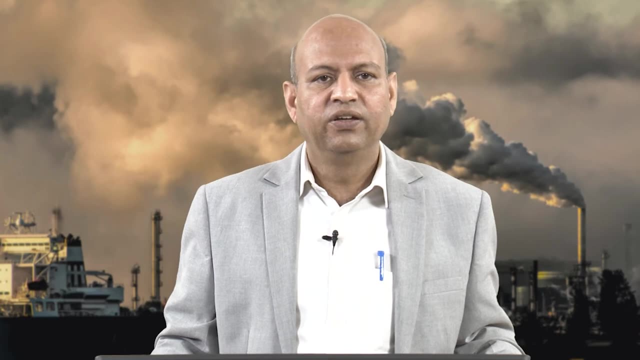 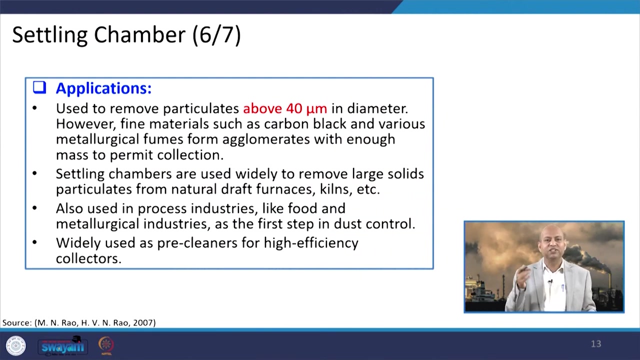 etc. Right Then. these settling chambers are used widely to remove Large solid particulate matters from natural draft furnaces, kilns etc. And also it is used, you know, in process industries like food and metallurgical industries, as the first step to dust control, as I said, so that the load on the secondary device can. 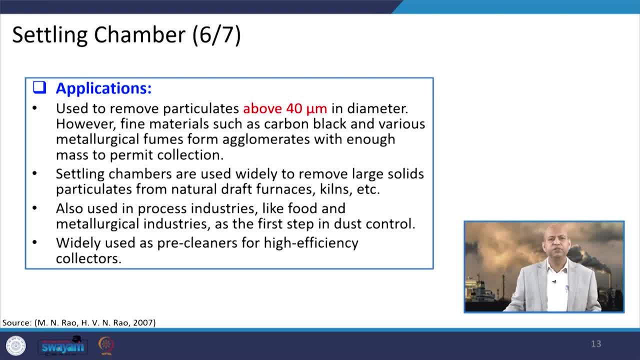 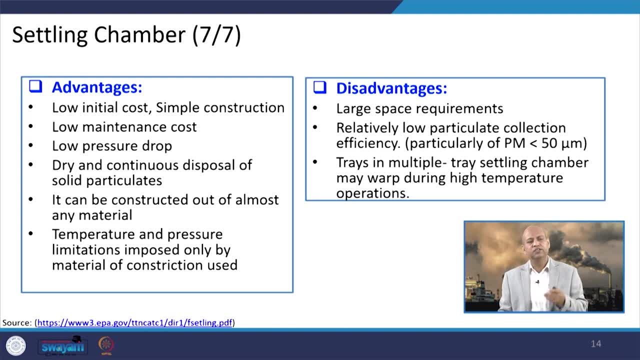 be reduced significantly And it is widely used, as pre you know, cleaners for high efficiency collectors. Then there are advantages and disadvantages. In advantages you can say that it is Low initial cost, simple construction. The construction is very simple kind of chamber you can provide. 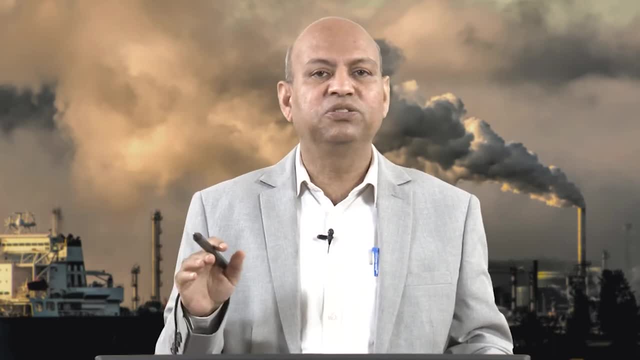 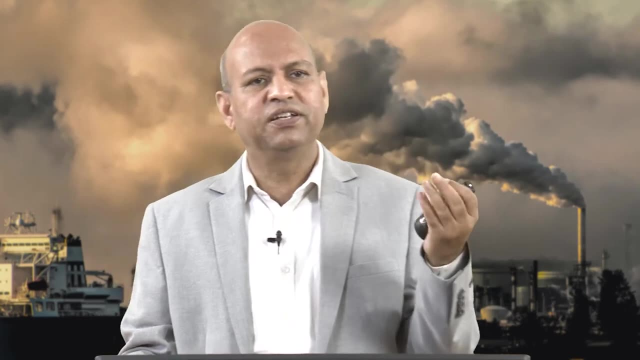 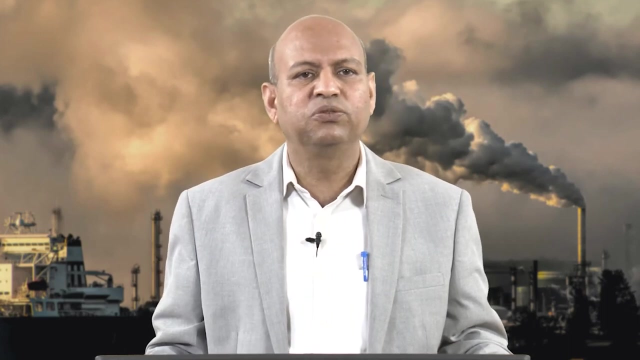 But you know, in terms of disadvantage you can say it requires large space. So in countryside it can be fine, but in urban areas it is difficult because land cost is much more. When we go for another, you know additional advantages, then you can say that it requires. 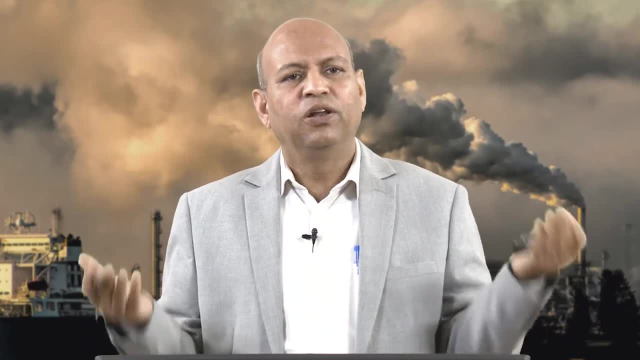 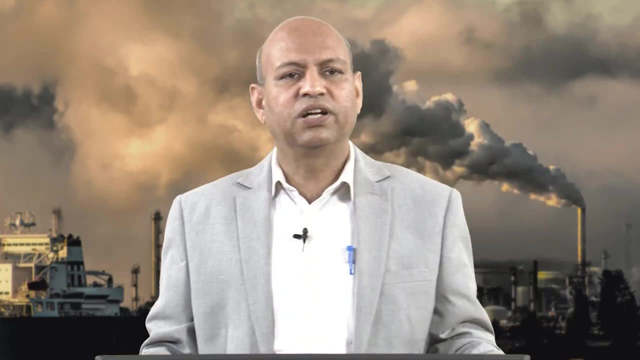 very low maintenance because there are no moving parts, etc. Low pressure drop is There, then dry and continuous disposal of solid particles can be achieved by these, you know, settling chambers, And it can be constructed out of almost any material, whether you construct by simple chamber. 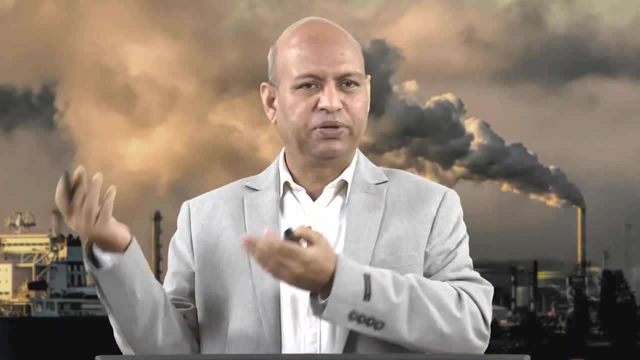 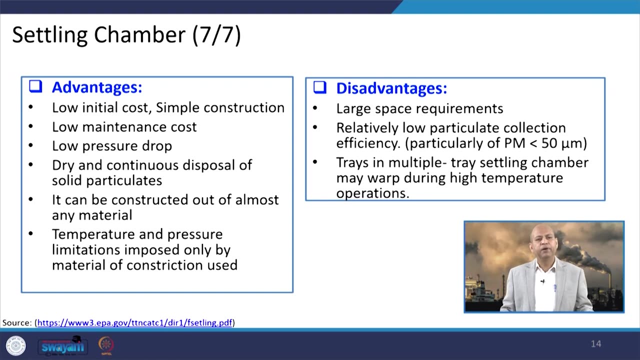 of some you know, metal or even bricks, etc. That is also possible. Temperature and pressure limitations imposed only by material of the construction use, So that way you can also control of which high temperature if you want to use, then according the material of those walls can be used. 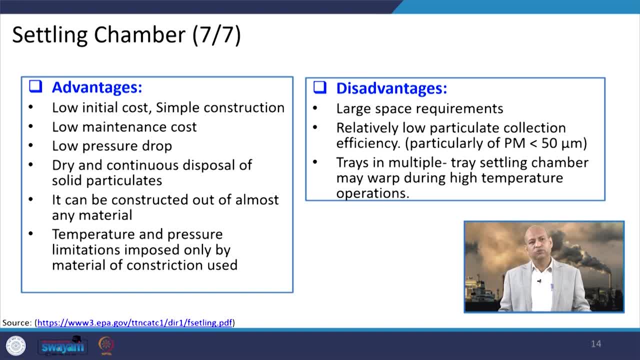 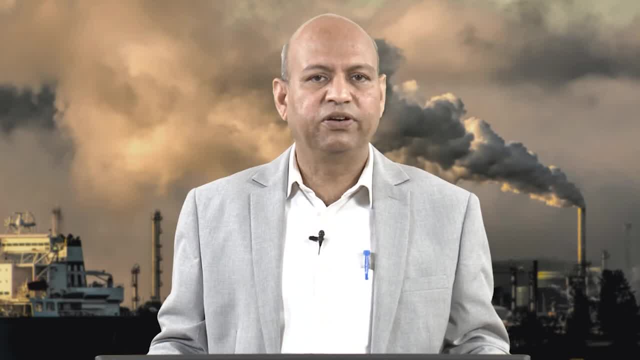 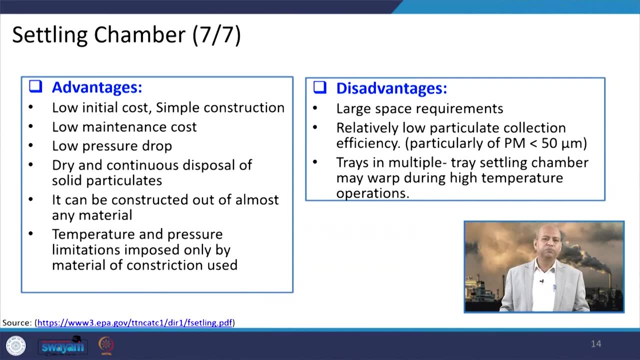 If you talk about the disadvantages, as I said, you know it requires large space So the land should be cheap in that particular location, otherwise it is not advisable. Then relatively low particle collection efficiency, like beyond 40 micrometer or 50 meter. if it is less than that then it is difficult to trap them unless we provide those horizontal. 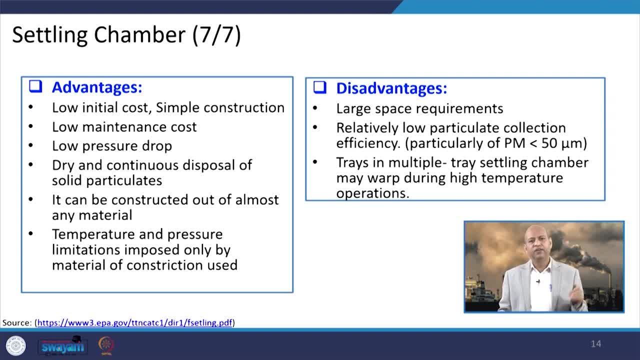 trays etc. It is good for 40 or 50 micrometer, Then trays in multiple. you know, tray settling chambers may warp during high temperature. They can undulate, They can, you know, get D shaped kind of things right. So those are the issues with this settling chamber. 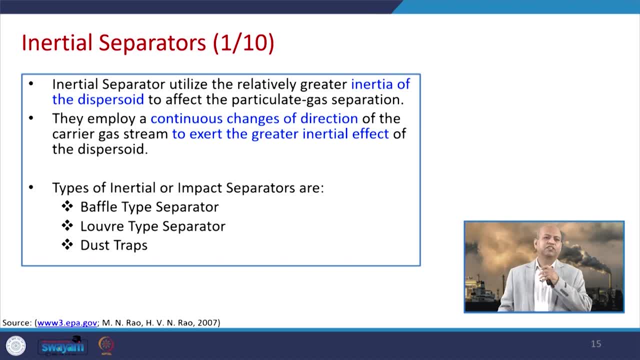 Then we come to the another device, which is known as inertial separators. So these inertial separators, basically, you know, utilize the relatively greater inertia of the these dispersal. So it is those fine particles to affect the particulate gas separation and they employ a continuous changes of the direction of the carrier gas stream to exert the greater inertial. 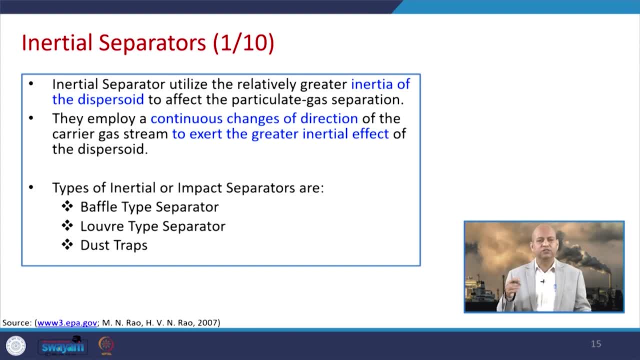 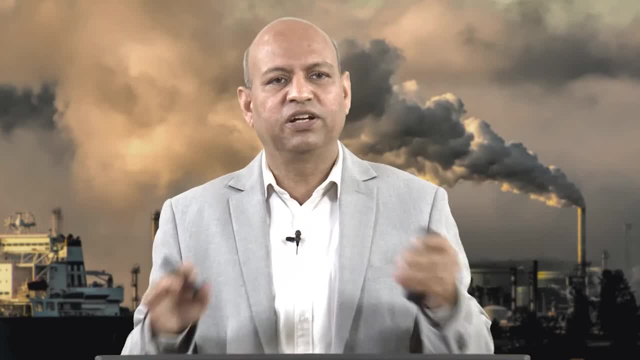 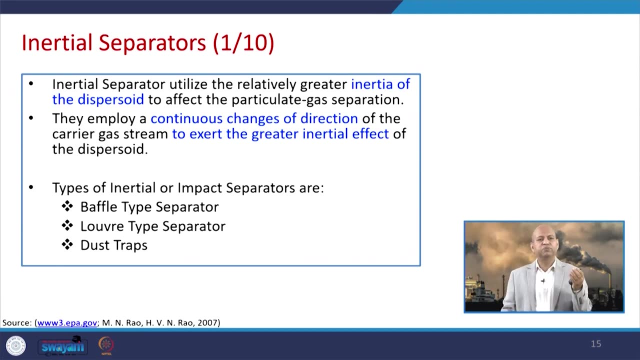 effect on the dispersal or particles, because impact will be more if we change its direction. we provide some, you know, baffle walls or those kind of things. So the types of inertial or impact separators can be like baffle type separators or lower type separators or dust trays. 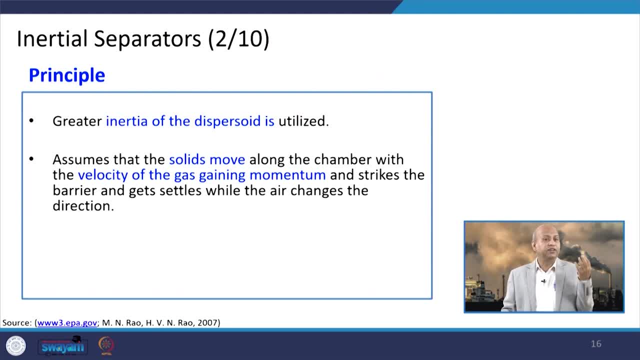 So we will see the principle, basically the inertia related. inertia: when, you know, you change the direction by baffles etc. Inertia occurs and they strike to the surface. then they lose the velocity and slide down And we this, you know these solid moves along the chamber with the velocity of the gas gaining. 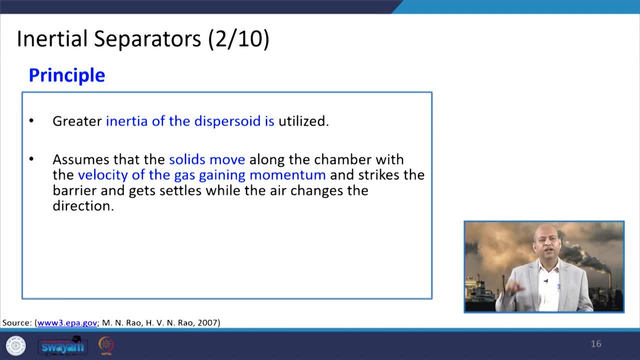 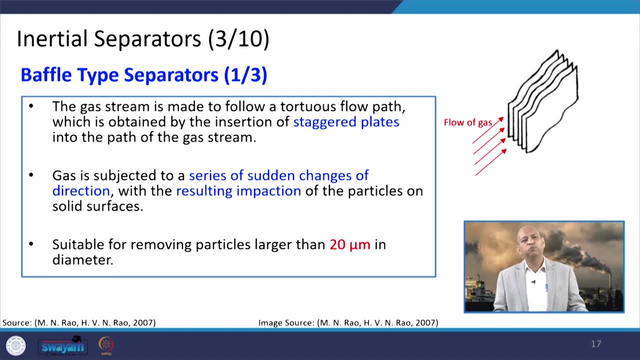 momentum and, as I said, it strikes at the barrier and gas settles down when air changes the direction because of losing the velocity. Okay, When we talk about baffle type separators, you can see these kind of. you know, there is kind of deformed kind of walls or we take, so that direction changes continuously right and the 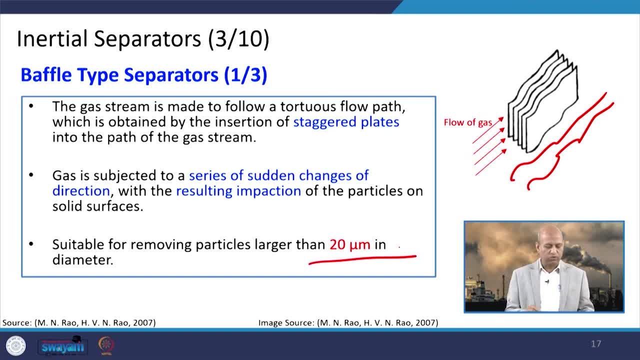 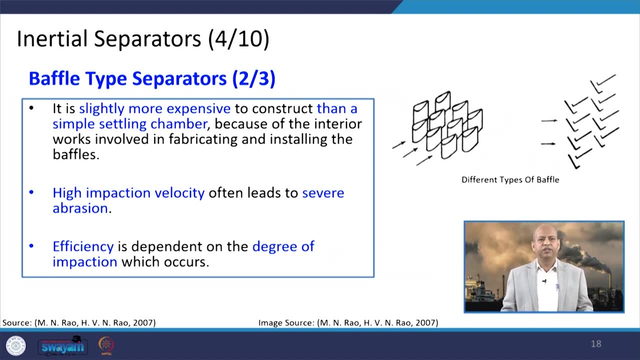 suitable for removing particles larger than 20 micrometer in diameter. So that way it is better if we compare with the settling chamber. Okay, So sudden change direction is to be ensured by these staggering kind of plates, etc. Well, you can see like, whenever you have a baffle type separator, you can see that the 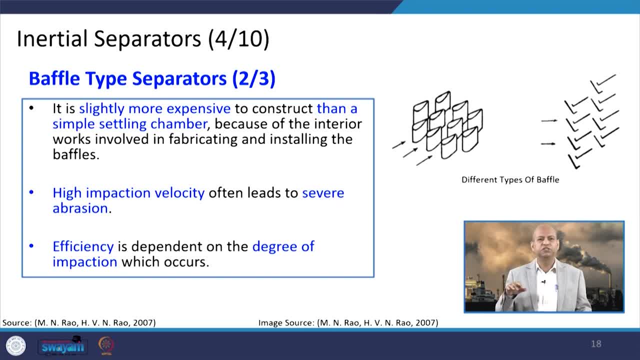 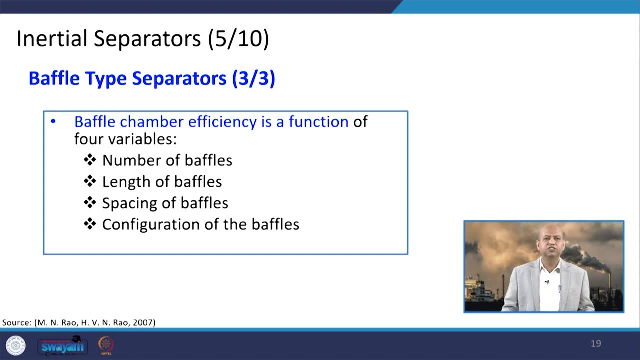 whenever these high impaction velocity often leads to severe abrasion. So those are the issues. basically, efficiency is dependent on degree of impaction which occurs. So those things we have to ensure if you want to remove more particles- And these you know, baffle chamber- efficiency is a function of four variables, basically. 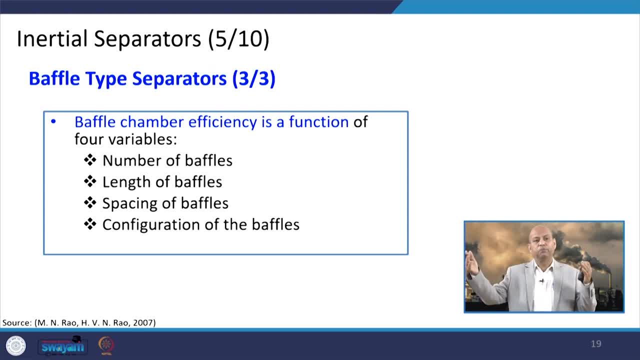 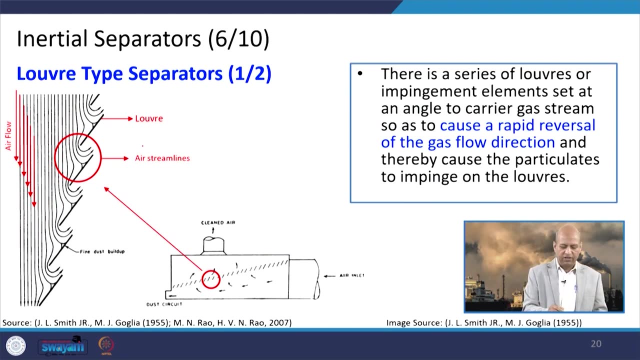 like number of baffles. we have provided length of the baffle, spacing of the baffle, configuration of the baffles, the types, etc. So these things, will you know, influence, As the you know, separation of the particles. basically You can see, like this louver type of separators, where these kind of louvers are installed. 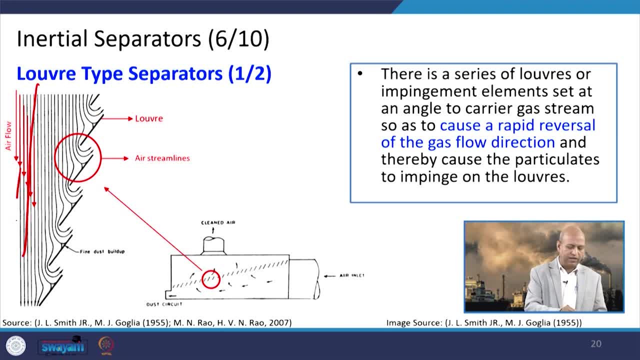 so that there is the change of the velocity, like air is going, like this, but nearer to these kind of you know insertions, this air changes its velocity and then this: it causes rapid reversal of the gas flow direction and thereby it causes the particulate matter to 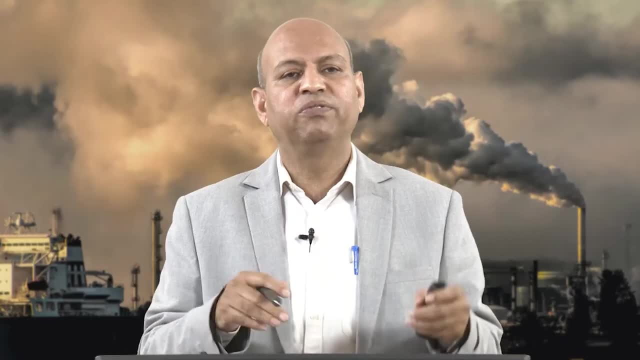 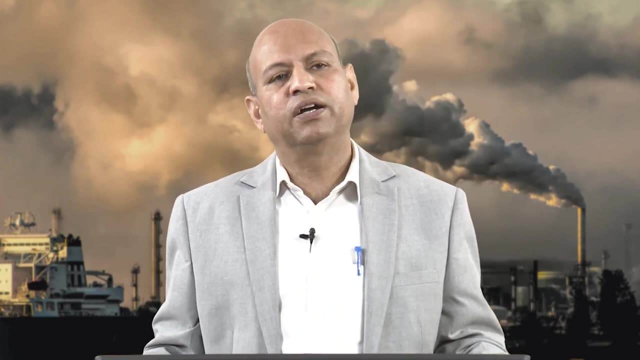 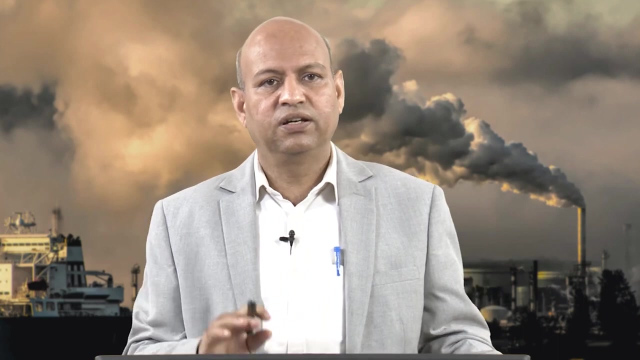 impinge on the louvers And lose the velocity and get down in the hoppers basically. So these type of louver type of separators can operate at the velocity of like 12 to 15 meter per second at the inlet. So that way you can, you know, have more efficiency. you can say: 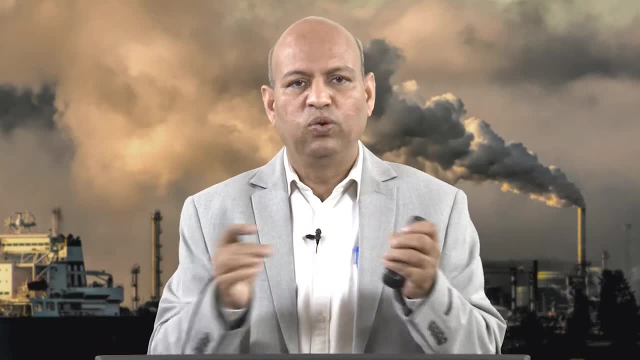 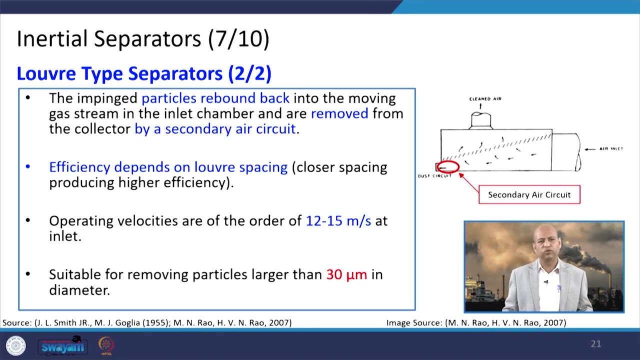 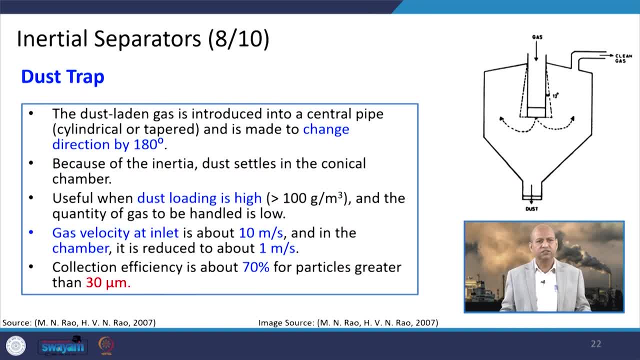 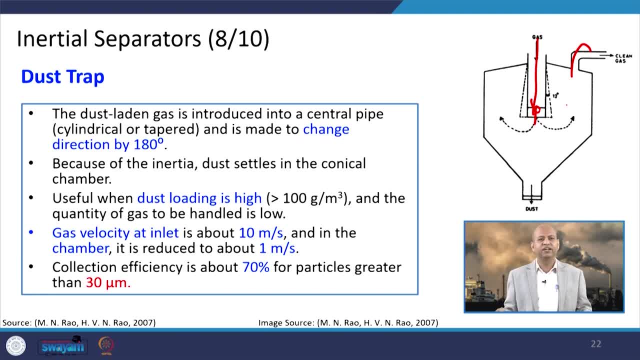 So it will go 180 degree. So in this change of the direction, it again, you know, have this tendency of striking to the walls and losing the velocity and getting down. And it is useful for dust loading when it is very high, like 100 gram per cubic meter. 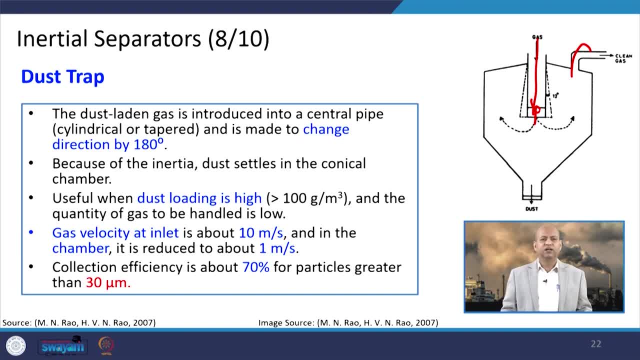 And this gas velocity at the inlet is like 10 meter per second in the chamber and it is reduced about 1 meter per second afterwards. Then again, collection efficiency is about 70 percent of the particles greater than 30 micrometer. So it is comparable with those earlier one. 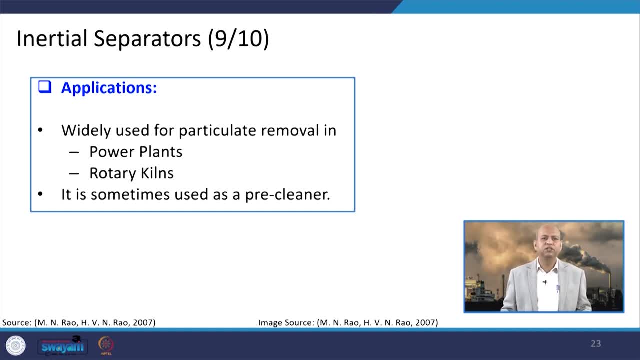 Then the applications of these inertial separators can be, you know, widely. it can be applied to the particulate matters removal, like in power plants Or rotary kilns, or it is sometimes used as the pre-cleaner as settling chambers also used, So that way also, these are devices which can be used for pre-cleaner before better devices. 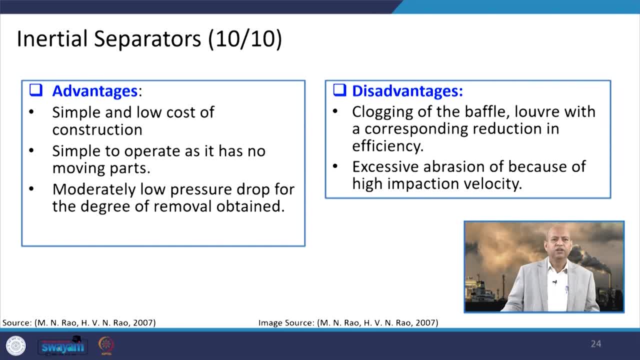 like ESP etc. Which we will see next. Then advantages and disadvantages. if we want to discuss about inertial separators, then advantages are like: it is again simple, low cost device and construction is also very easy. Simple to operate as it has no moving parts. 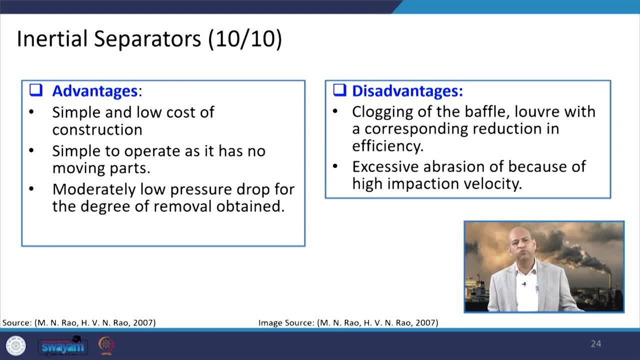 Then moderately low pressure drop for the degree of removal obtained. but there are disadvantages like clogging of the baffle walls or louver, with the corresponding reduction in efficiency occurs after some time. So you have to clean that after some time. Then excessive abrasion because of high impaction velocity also occurs. 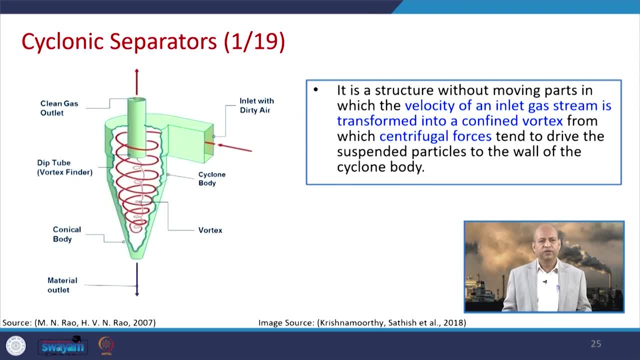 So maybe you have to change those baffle walls or louver kind of structures. Now we come to the cyclonic separators. So in cyclonic separators, Basically it is nothing but a structure without moving parts in which the velocity of an inlet gas stream is transformed into a confined vortex, that circular motion from which centrifugal 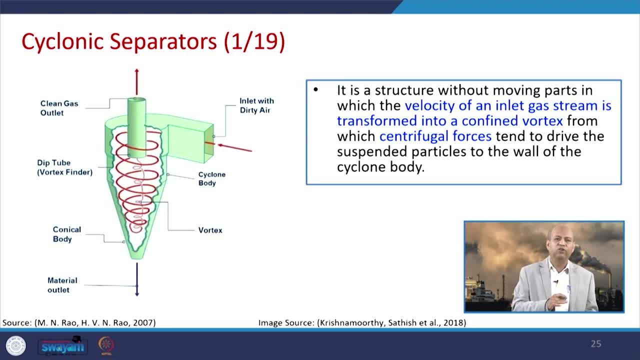 forces tend to drive the suspended particles to the wall of the cyclonic body. So like, for example, this inlet is there and this gas goes downwards. basically, it goes downwards in circular motion, right So in circular motion because of centrifugal force, The tangential force it restricts to the wall and loses its velocity and gets down the hopper. 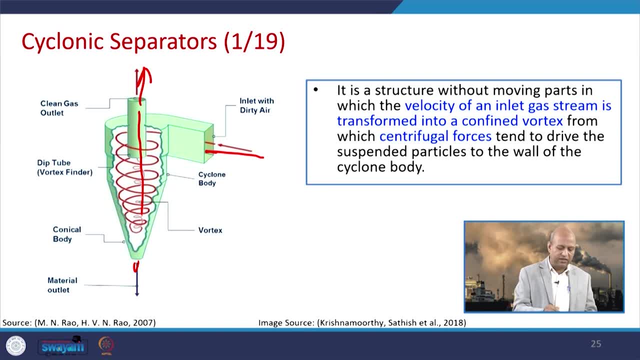 Then when it goes up- because outlet is in this direction, So it goes up again in circular motion- it goes there also again. it is trapped and whatever remaining particles- smaller particles they can be- again give their velocity to zero and come down. So that way cyclonic separators work. 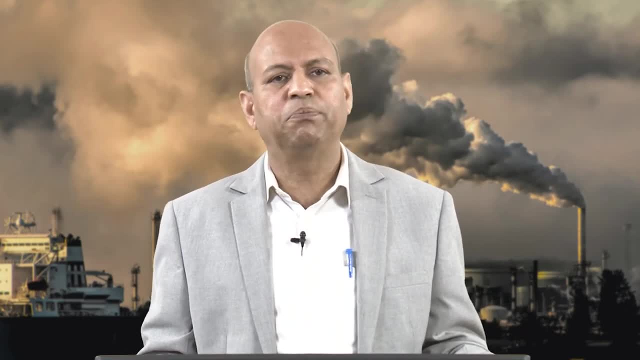 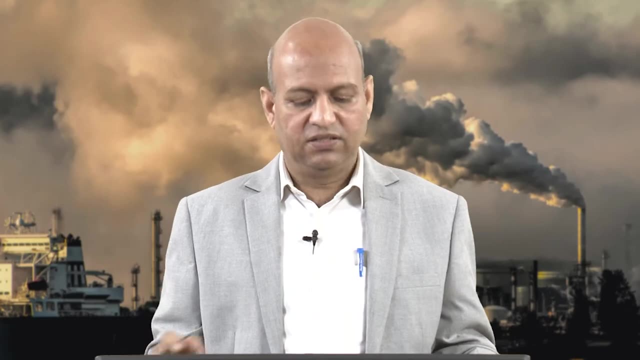 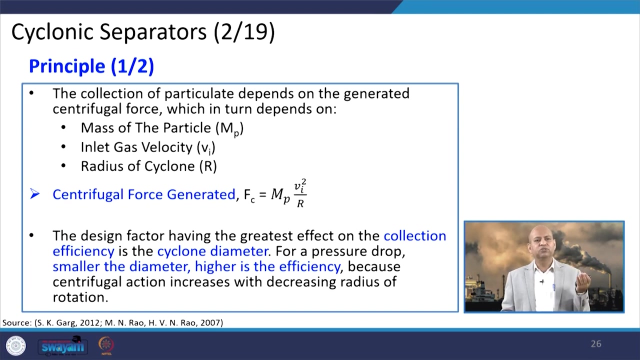 So its principle basically, have you know: influence of the mass of the particles, inlet gas, velocity or radius Of the cyclone. because the centrifugal force generated is like this: m p into v, i square upon r, where mass of the particle is m p and the radius of cyclone is r and the inlet gas 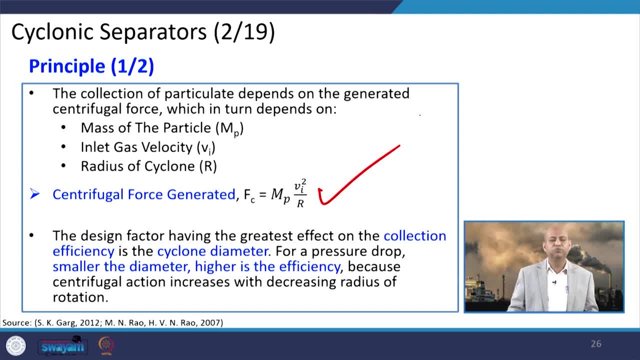 velocity is the v? i. So this particular, you know, relationship will work to get the particle separate from the cyclonic separators and the design factor you know having the greatest effect on the collection efficiency is the cyclone diameter. basically, Okay, This radius you can. 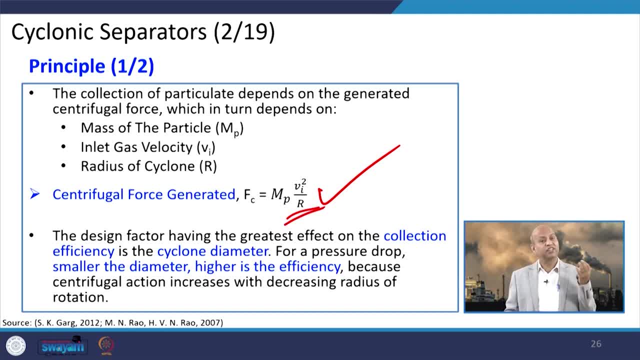 Say, for a pressure drop is smaller the diameter, higher the efficiency. Okay, Because centrifugal action increases with the decreasing radius of the rotation, because it is in the denominator Okay. So that is the very simple thing you can see like this principle: again, the minimum diameter: 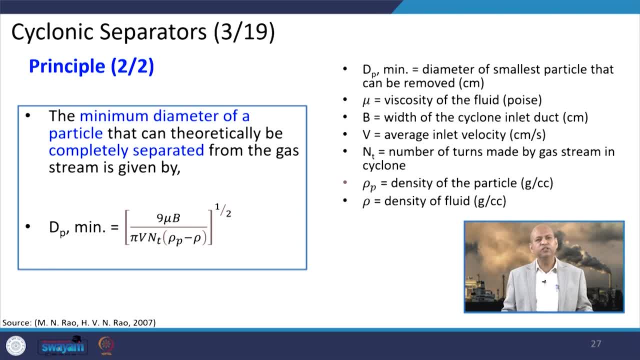 if you want to calculate for a particle that can theoretically be removed completely from the cyclonic separator, then this is the relationship. dp can be calculated by this equation: 9 mu b divided by pi, v, nt, rho, p minus rho, where dp is the minimum diameter of the smallest. 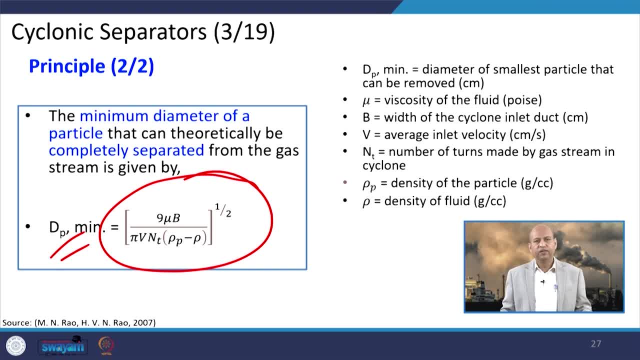 particle which can be removed by this particular mechanism. Mu is the viscosity of the fluid that is the gas also- and the b width of the cyclone inlet duct- Okay, When it is coming Right. And then the v is the average inlet velocity and t is the number of tons made by gas stream. 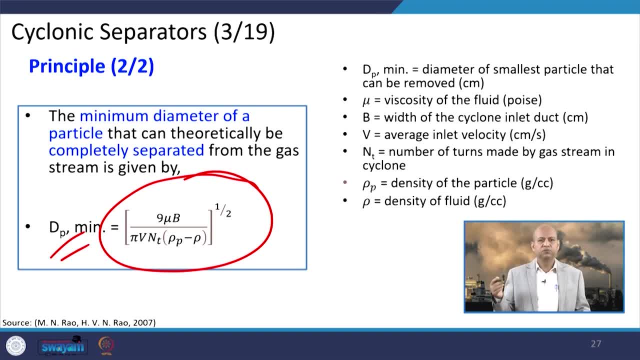 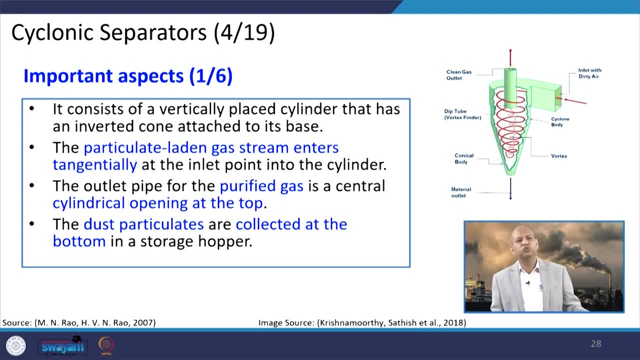 in the cyclone when it comes down And go up. So rho p density of the particle, so is the density of the fluid. Important aspects: like you know, it consists of vertically placed cylindrical, you know apparatus that has an inverted cone, kind of attached to the base. 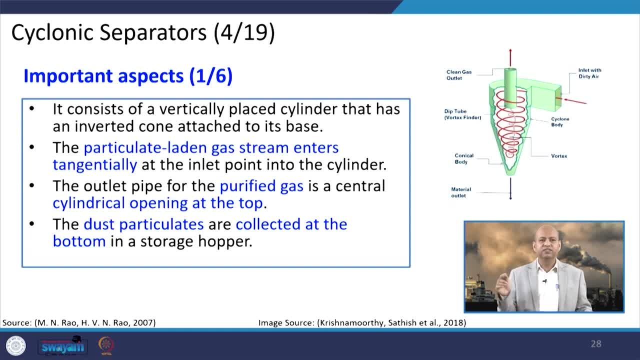 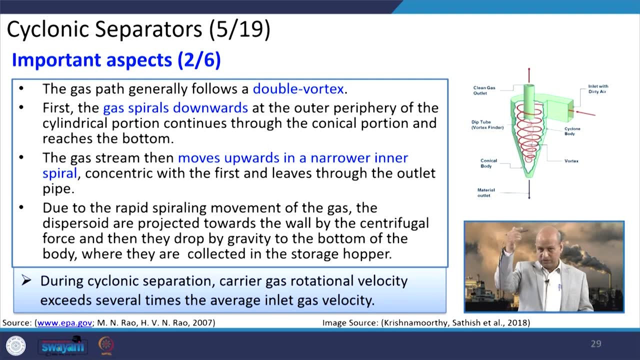 And the particulate laden gas stream enters tangentially, as I said earlier, at the inlet point here Right, And then it goes down And the dust particles are collected at the bottom in the storage hopper. Okay, The gas path generally follows a double vortex, as I said. once it comes down, then it goes. 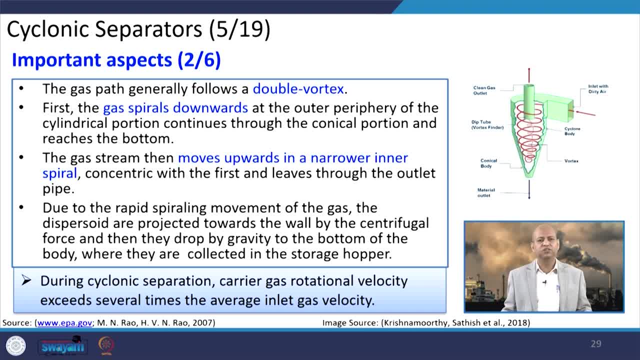 up inside. So double path is there. So that way, you know, there is a possibility of, you know, collection of smaller particles also And the, during cyclonic separation, carrier gas rotationally. you know rotational velocity exceeds several times the average inlet gas velocity. So that is the, you know, very important point you can see for removal of these particles. 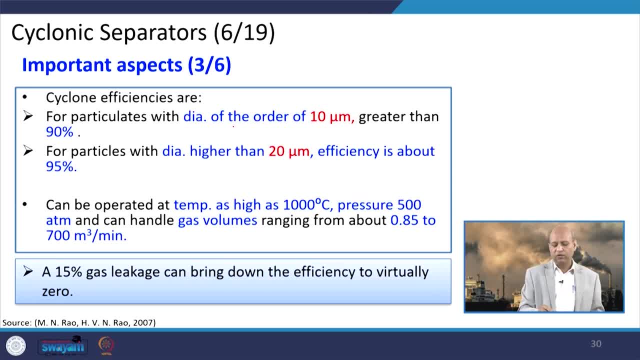 So cyclone efficiencies. Efficiencies are like for particulates of the order of 10 micrometer or so, greater than 90 percent. If particles are of the size of 20 micrometer or so, then efficiency further increases 95 percent Right. 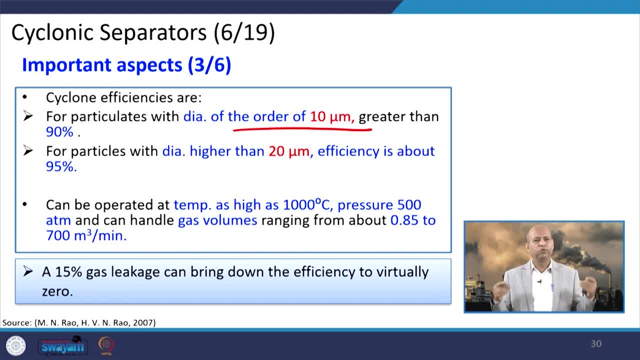 So more coarser particles. naturally, mass is more, removal efficiency is more And it can be operated at the high temperature like 1000 degree Celsius pressure of the 500 atmospheric pressure. It can handle gas volumes ranging from 0.85 to 700 cubic. 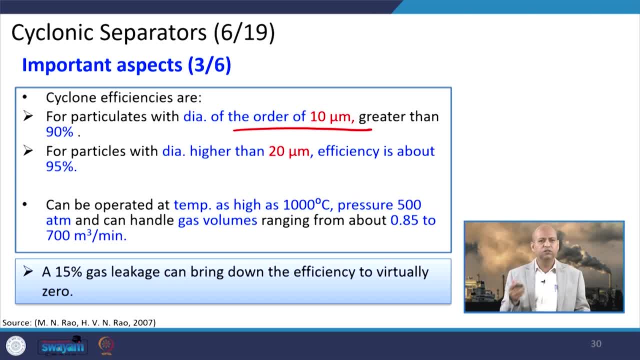 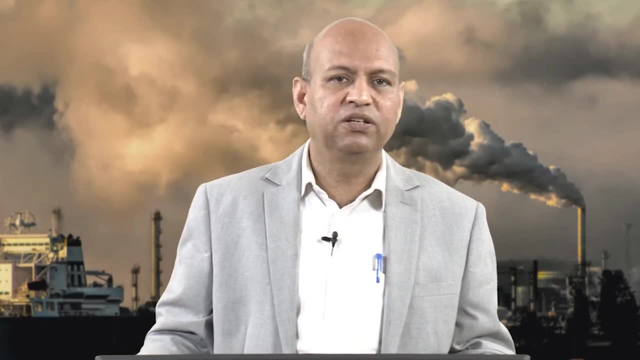 meter per minute. So means good flow rate can be handled. A 15 percent gas leakage can bring down the efficiency to virtually 0. So the leakage should not be there. That is very important aspect in this case. So wherever leakage, it should be handled properly and promptly, otherwise efficiency will be. 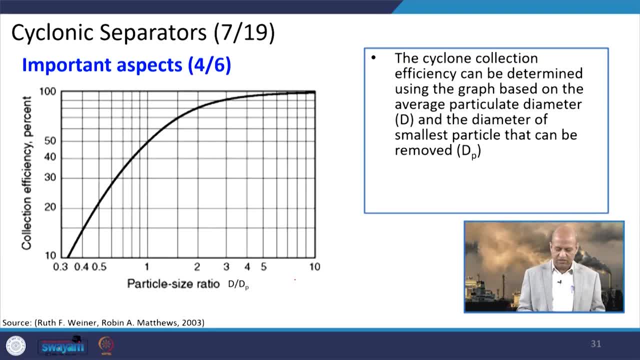 drastically reduced. In this you know graph you can see the. you know efficiency: collection efficiency depending upon the size of the. you know this ratio of the particle, This ratio of the particle, This d and dp. particular diameter: d and diameter: smallest particle that can be removed: dp. 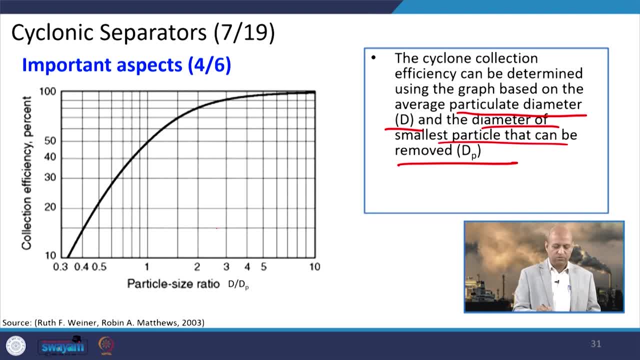 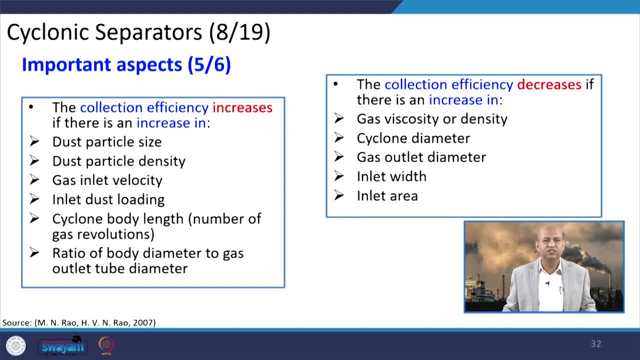 So if it is like 10 up to 100, it can be removed. So you can see the ratio and you can decide the efficiency. Well, the important aspects like the collection efficiency increases if there is an increase in, like dust particle size or dust particle density or gas inlet velocity or inlet dust. 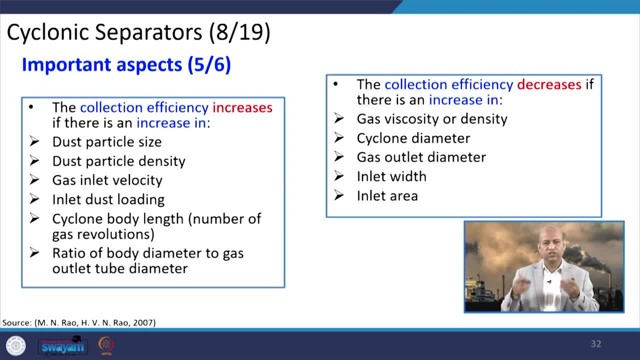 loading or cyclone body length. number of gas revolutions, because it will ensure more gas. these revolutions, Then ratio of the body diameter to the gas outlet tube diameter and the collection efficiency decreases with the gas. viscosity or density or cyclone diameter or gas outlet diameter, inlet width or inlet area. 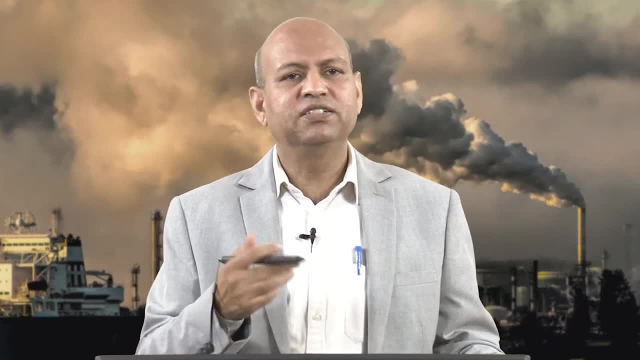 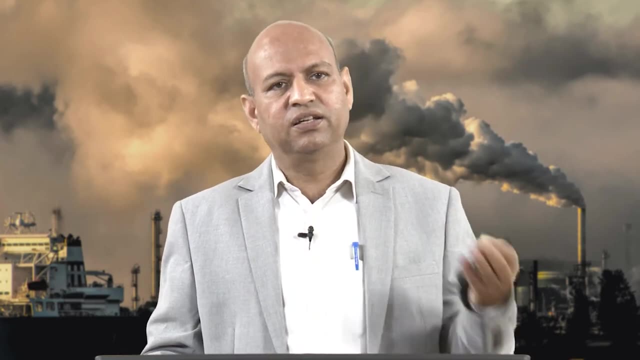 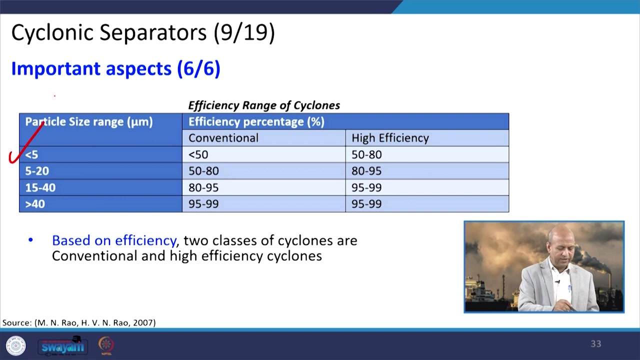 So these very kind of thumb rules, you can see, these aspects can be observed or taken care when we want to design cyclonic separators. and then another you know set of important aspects are there, Like: So the size of the particles: are there less than 5 micrometer, or 5 to 10,, 15 to 40 more? 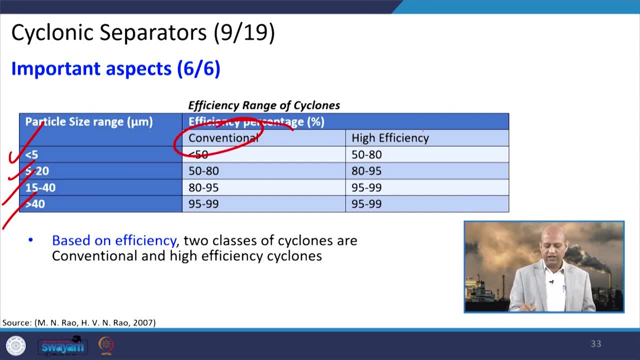 than 40. Efficiency. you know conventional and high efficiency kind of separators may be there. So in conventional, like for less than 5, less than 50 percent efficiency is there. high efficiency can ensure 50 to 80 also, And you know, like 40 micrometer or so, 95 to 99 in conventional and in high efficiency. 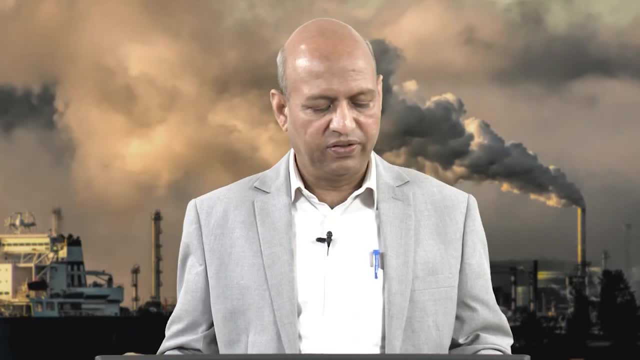 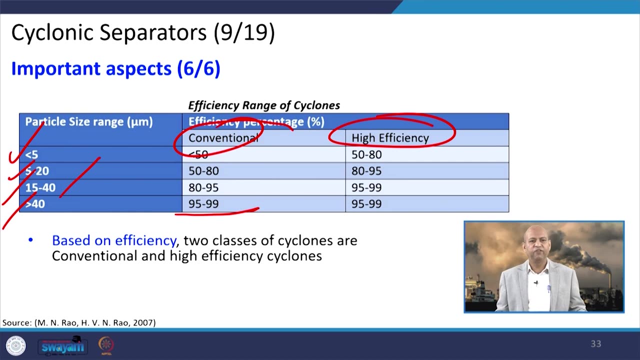 also. So the limit, you can say up to the 40. Otherwise, the basic thing is difference in this 5, 20 and, you know, 15, 40. that is the efficiency difference. And based on the efficiency, two classes of cyclones have been, you know, categorized like: 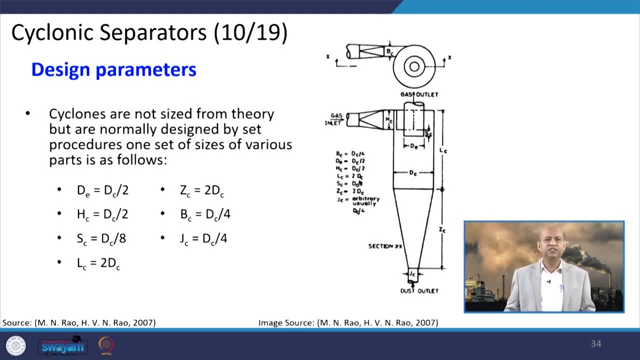 conventional and high efficiency. If you want to see the design parameters, basically, you know, based on you know, several design exercises or practices or observations, there are certain, you know, relationship, empirical relationships which have been decided like this: DE equals DC upon 2, ZC equals DC upon. 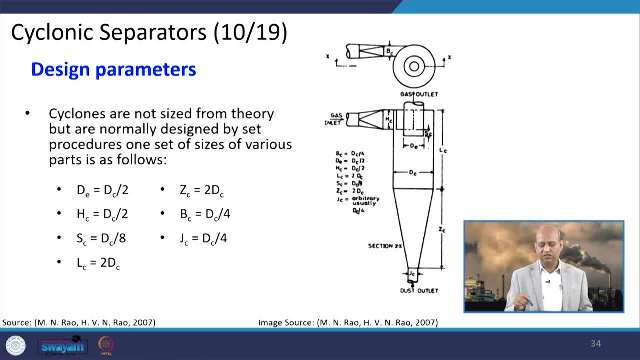 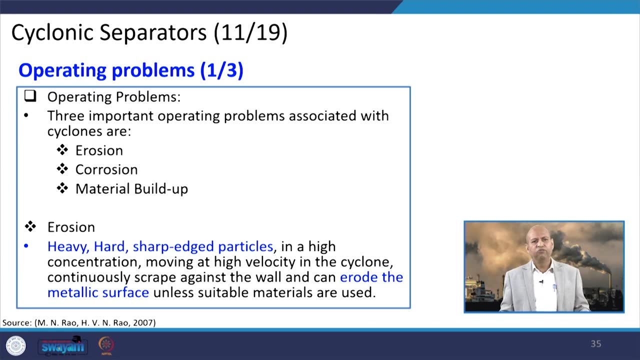 2.. So these are the you know dimensions you can see in this cyclonic separator cross section and those particular relationships are, you know, taken into consideration when we design So that become, you know, better or efficient way of designing. Well operating problems are there. 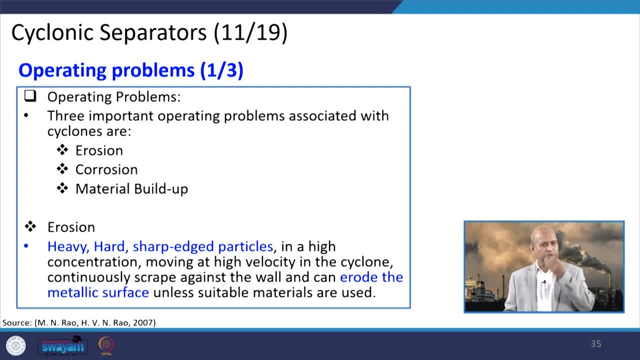 Like It can eroded by particulate matter because it strikes to the surfaces, Corrosion may be there. if those you know gas carrier gas is having like acidic content, like SO2, etcetera, Then material buildup can be there at the you know inlet, outlet or some surfaces also. 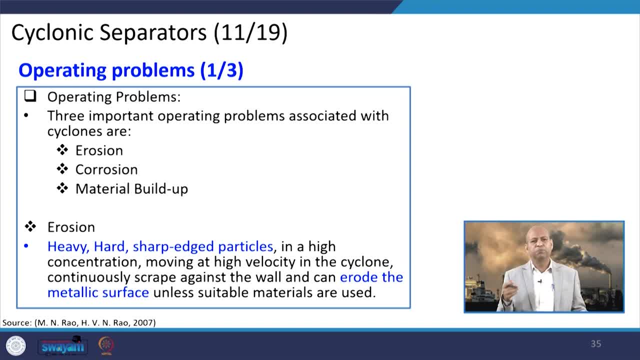 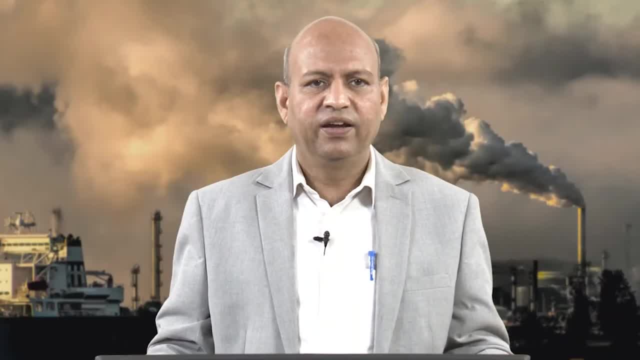 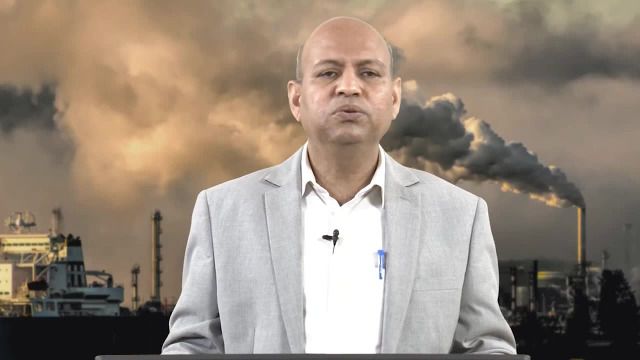 So you know, at some surfaces sometimes people use those kind of like rim kind of thing and it can be removed. Otherwise regular cleaning is needed. So needed And corrosion related means you have to see that the carrier gas is taken into at the temperature where dew point is not achieved. only then it would be better, otherwise corrosion. 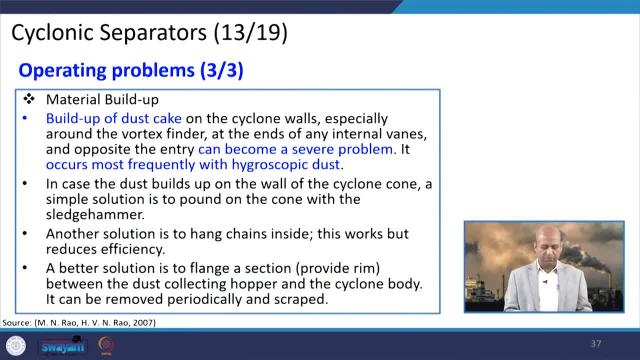 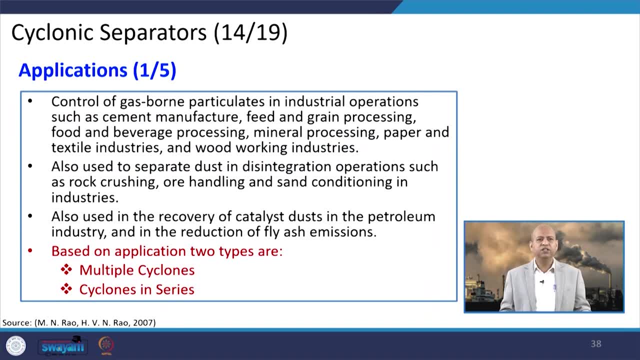 problem may be there And, as I said, material buildup can be taken into consideration and it can be removed by this rim provision or by regular cleaning. Well, applications can be there in many cases, like it can be used as the multiple cyclones or cyclones in series, depending upon. 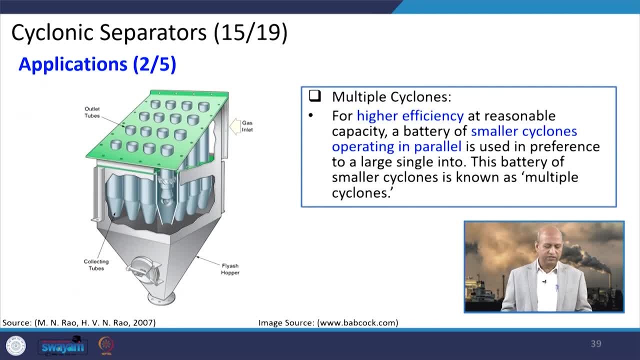 what kind of pollution load is there, For example, to increase the efficiency in row and parallel rows as well? as this kind of system may be there where smaller cyclones can be put together and multiple cyclones, we can call it, so that more cyclones are available to remove. 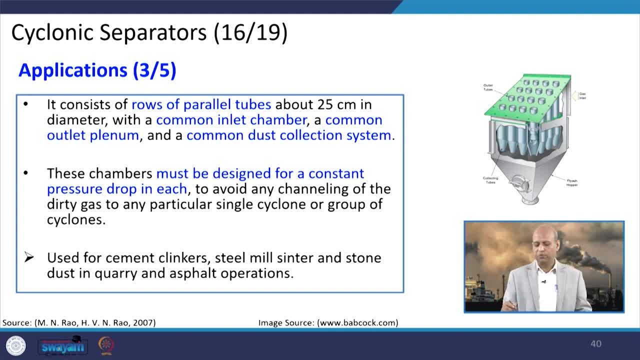 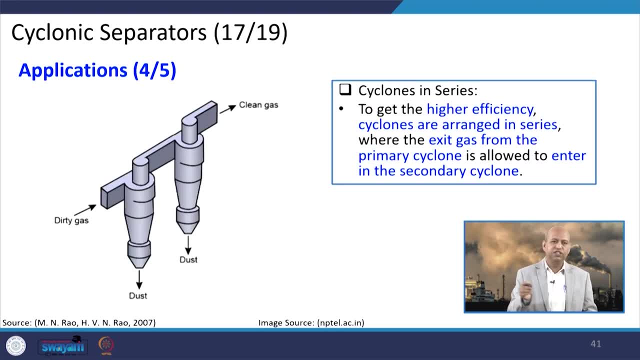 the particles. Well, this can consist of different rows, two or more, And depending upon their distance and collection, efficiency can be calculated. If we go into series, only one after one, then dirty gas goes to one particular this separator, then more cleaner gas. 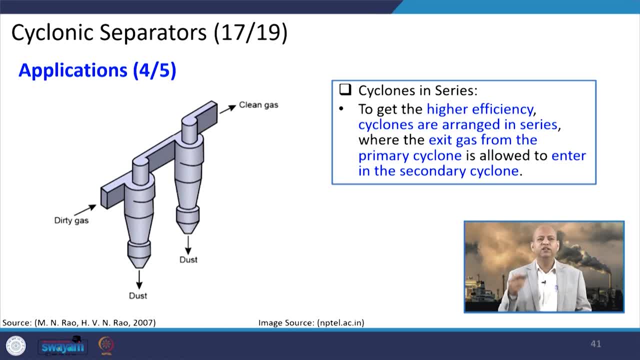 goes to another separator. That way, you can ensure very high efficiency or very clean gas at the outlet, depending upon how many cyclone separators you have installed in series, basically. So if you want to do that, then you can do that. So if you want to do that, then you can do that. 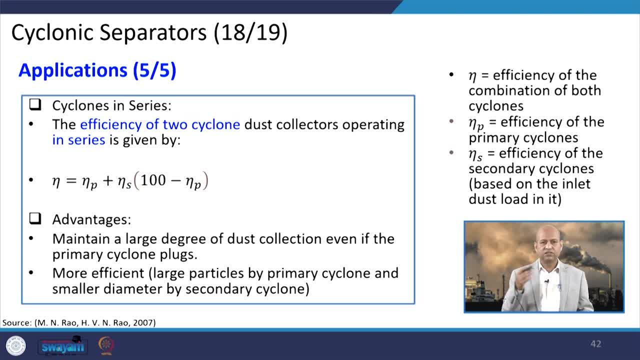 So if you want to calculate the efficiency in cyclones installed in series, then this is the simple formula like: eta equals eta p plus this, eta s, 100 minus np. So this is basically this eta efficiency of the combination of both the cyclones. eta p is efficiency of the primary. 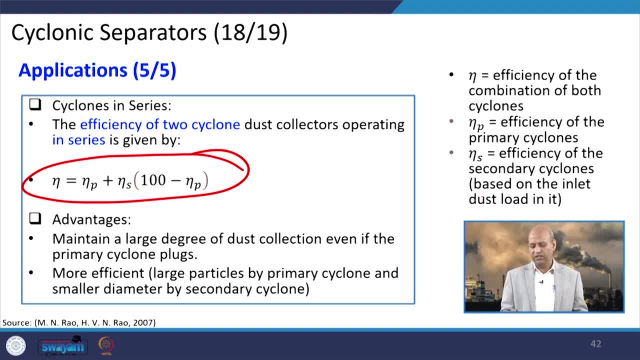 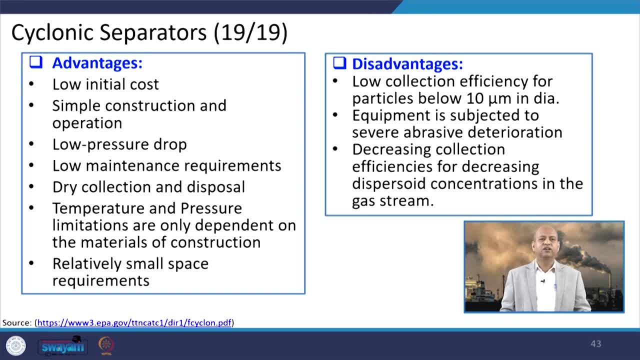 cyclone. that is initially. then efficiency of the secondary cyclone, based on the inlet dust load in it, So that can be used. Then. advantages are like low cost, initial low cost, simple construction and operation, low pressure drop or low maintenance. 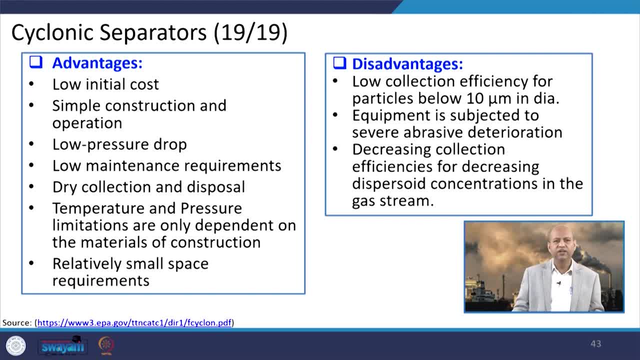 requirement. dry collection and disposal is very easy. Temperature and pressure limitations are only dependent on the materials of the construction, So that way you can have different kind of material. if there are issues with the temperature, Relatively small space required because vertical you can design it, So horizontal space may not be a big problem, which is problem. 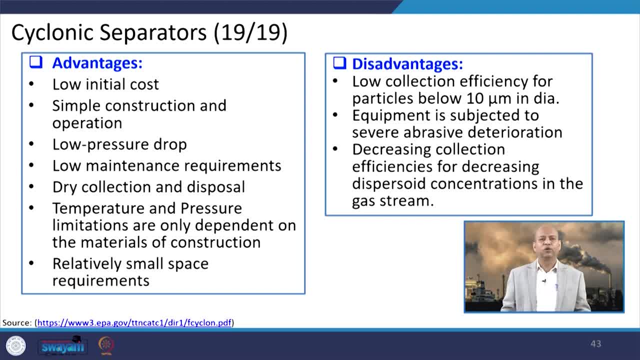 in the settling chamber. Disadvantages like low collection efficiency for particles below 10 micrometer in diameter. Equipment is subject to the severe abrasive deterioration depending upon the particle size, its sharpness, etc. Then decreasing collection efficiency for decreasing dispersoid concentration in the 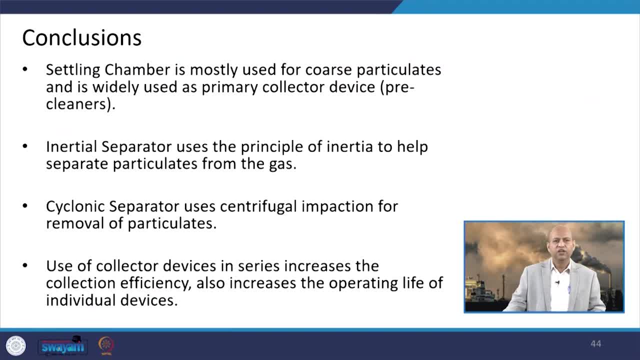 gas system. So those are the issues of the disadvantages. Well, so overall we can say that the settling chamber is mostly used for coarser particles, because it is very simple device. it works on gravitational force, So there is no other external forces we are using. So